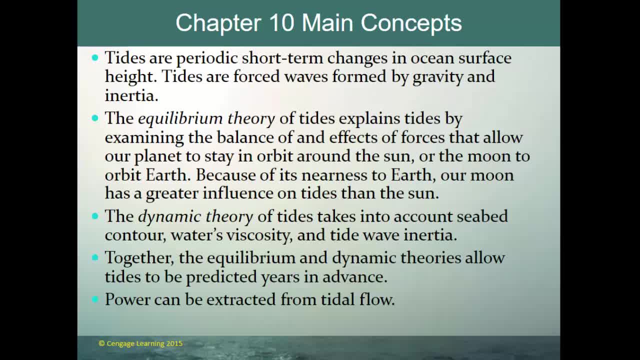 Together, the equilibrium and dynamic theories allow tides to be predicted not only for tomorrow, but actually years in advance, And one of the great things about tides, other than knowing when high and low tide, will be to know when the best surface is going to be. you can also extract power from tidal flow. 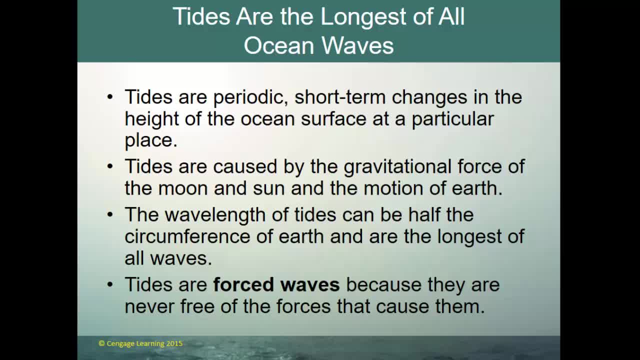 Alright, so tides are the longest of all ocean waves. Periodic short-term changes in the height of the ocean surface at a particular place, Caused by the gravitational pull, The gravitational force of the moon and sun and the motion of the earth. 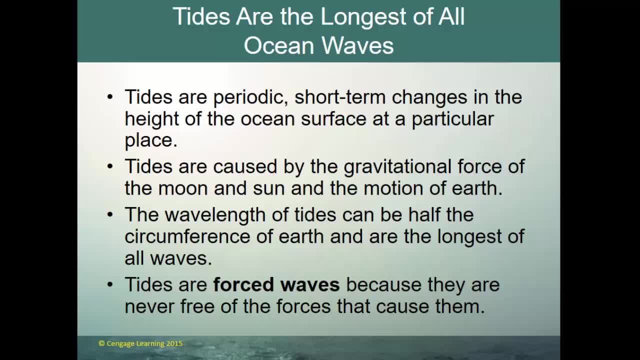 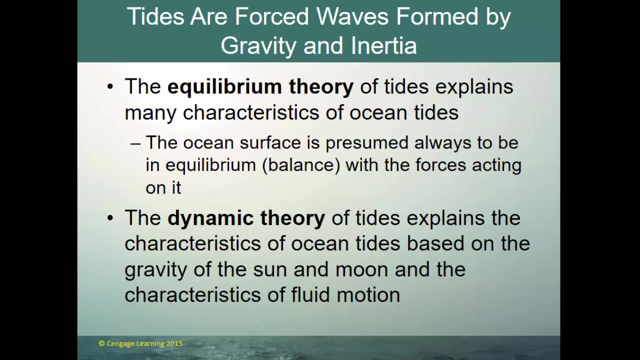 The wavelength of tides can be half the circumference of earth and are the longest of all waves. Tides are considered forced waves because they are never free from the forces that cause them, specifically never free from gravity. The equilibrium theory of tides explains many characteristics of ocean tides. 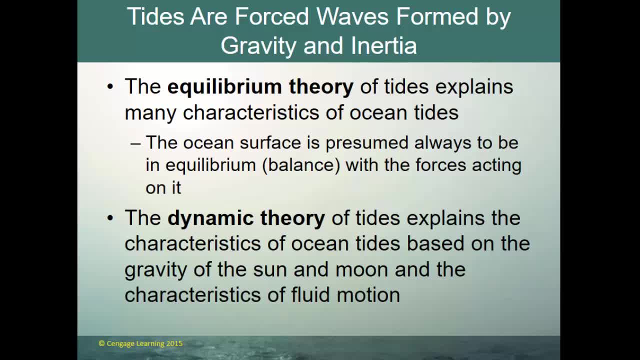 The ocean surface is presumed always to be in equilibrium, that is, in balance, With the forces that are acting upon it. The dynamic theory of tides explains the characteristics of ocean tides based on the gravity of the sun and the moon and the characteristics of fluid motion, and also the seabed in the shape of ocean basins. 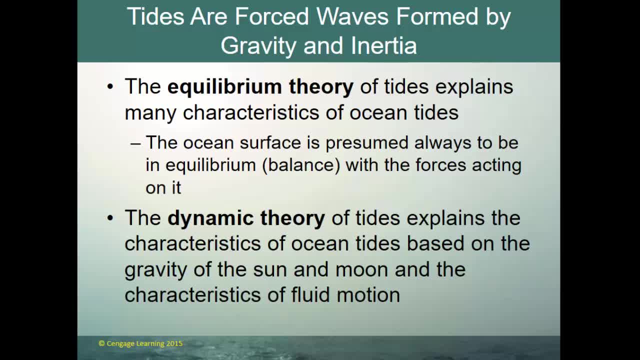 And the shape of the basins that tides are acting in. So the equilibrium theory again, basically, is looking at the gravitational forces playing to force the waves. The dynamic theory takes in to all the other subtler aspects And that dynamic theory makes tide calculations. 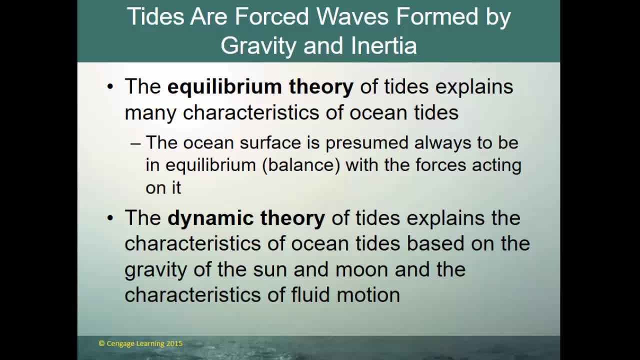 calculations a very complex thing. It's not a simple thing at all. Very, very complex formulas go into it, But once those formulas are solved we essentially can know the tides for years into the future. Gravity, as we know, holds bodies together. A planet orbits the sun in balance. 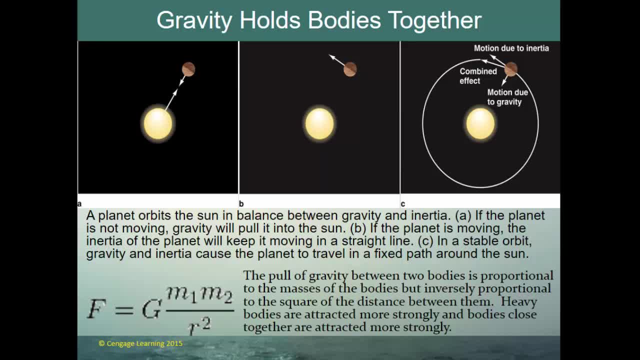 between gravity and inertia. If the planet is not moving, gravity will pull it into the sun. If the planet is moving, the inertia of the planet will keep it moving in a straight line In a stable orbit. gravity and inertia are in balance and cause a planet to travel in a fixed 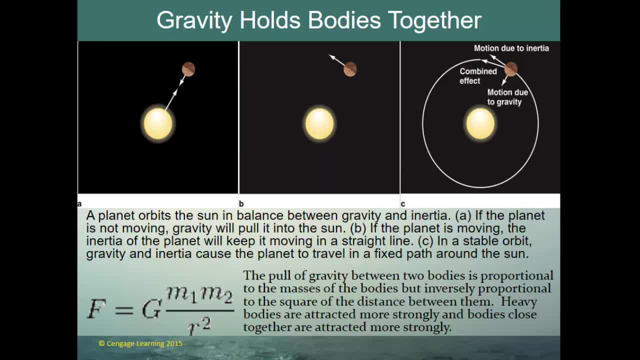 path around the sun. So A- you have a non-moving planet being pulled toward the sun, and B- you have a planet that is moving in a direction, in a straight line- And, of course, remember that bodies tend to move in a straight line unless another force of acceleration acts upon them. 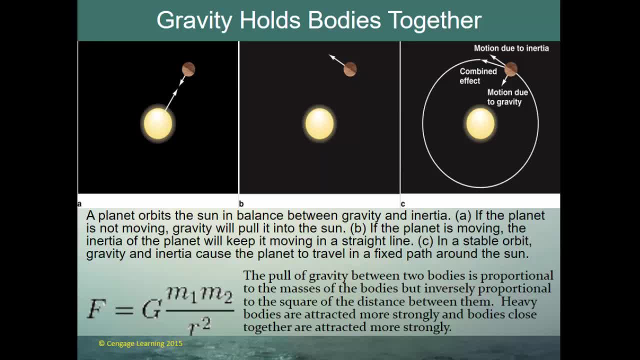 And so the gravity is that other force causing the motion of the planet to be in not necessarily a circle, but more like an ellipse around the sun. So the pull of gravity between two bodies is proportional. Now, this is what the force of gravity is. Pull of gravity is: 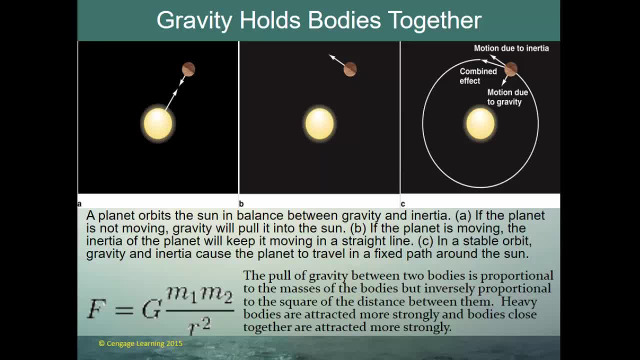 proportional to the masses of the bodies, that's m1 and m2,, but it is inversely proportional to the distance between them. Hence, heavier objects generate more gravity, and the further the distance between two objects, the less gravity there's going to be. Heavy bodies are attracted. 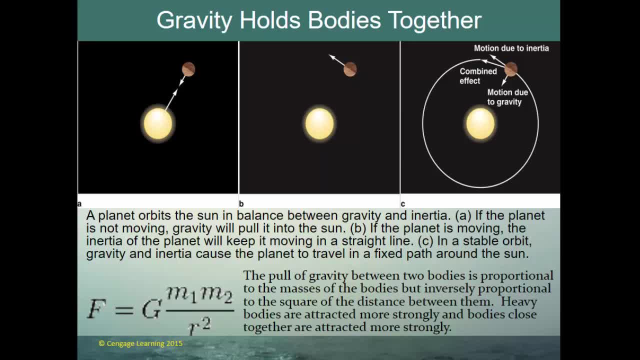 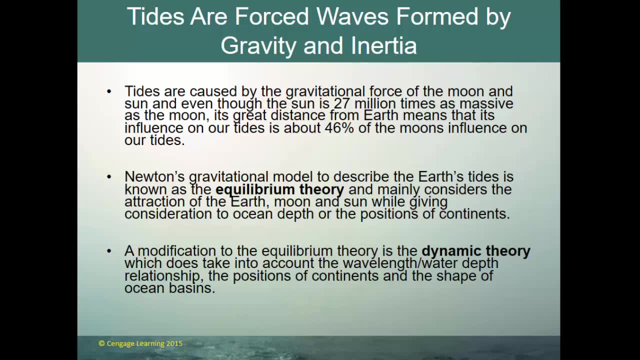 more strongly than bodies, And bodies close together are attracted more strongly. So tides again are forced waves formed by gravity and inertia. Tides are caused by the gravitational force of the moon and the sun, and even though the sun is 27 million times as massive as the moon, its great distance, 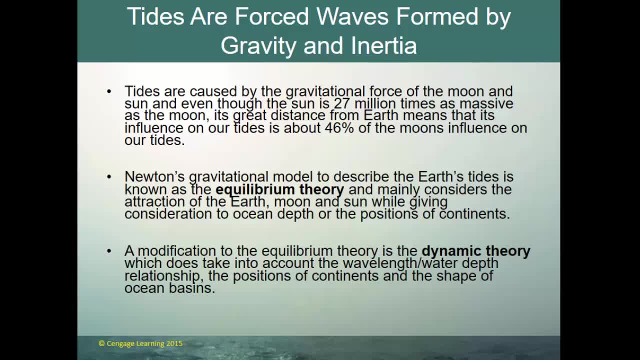 from the earth means that its influence on our tides is about 46% of the moon's influence on our tides. That doesn't mean the moon exerts 54% and the sun exerts 54% of the sun exerts 46%. That means the power that's exerted by the moon. the sun's influence is only 46% of that. 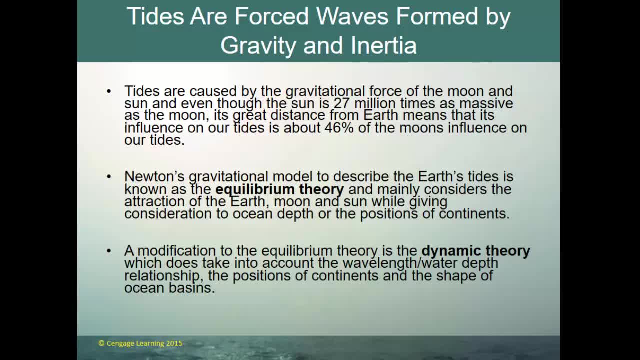 Newton's gravitational model to describe the earth's tides is known as the equilibrium theory and mainly considers the attractions of earth, moon and sun, while giving some consideration to ocean depth or the position of continents. The modification to the equilibrium theory is that 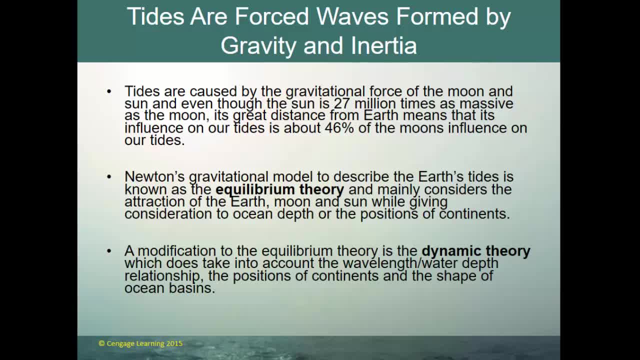 dynamic theory, which does take into account the wavelength of the wave, the water depth relationships, the positions of the continents, ocean basins, the density of water, the seafloor topography, or what's known as bathymetry, and lots of other very subtle. 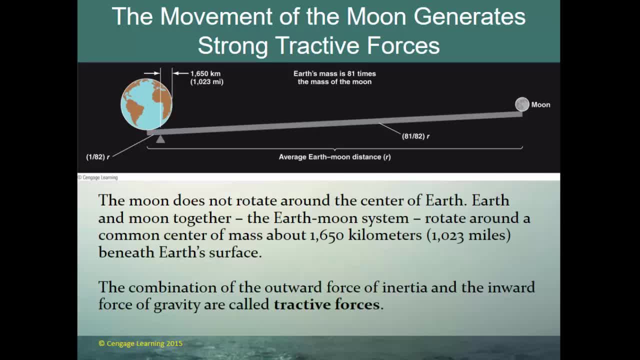 effects that change how tides work in different basins. The movement of the moon generates what's known as strong tractive forces. So in this example we see the distance between the earth and the moon and the mass of the earth being 81 times the mass of the moon. 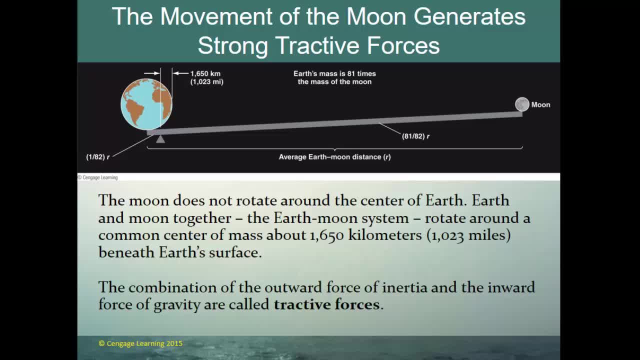 and what we know, then, is that the pivot point around which both the earth and the moon spin is this point, just inside the earth's surface. So the moon does not rotate around the center of earth. The earth and the moon together create the earth-moon system, and they rotate around a common center. 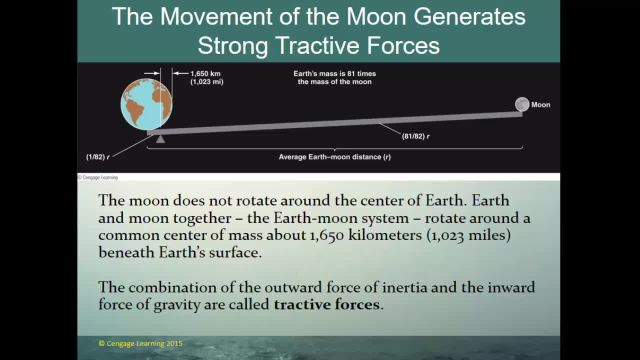 So the common center is that. the common center of mass is that point about a thousand miles beneath the earth, the earth's surface. That's where that fulcrum of that lever is. They're just about a thousand miles inside the earth's surface. So the combination of the outward force of inertia- remember the moon- 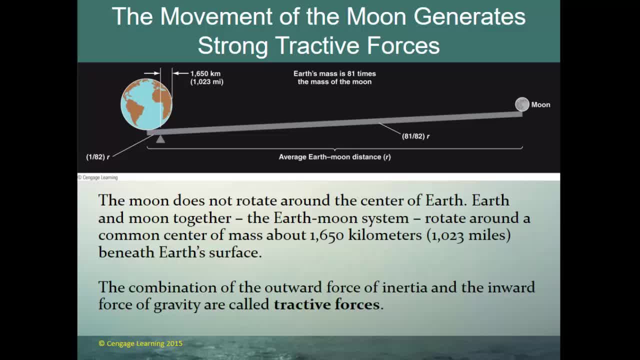 is moving in a straight line and the inward force of gravity are known as the tractive forces. So we can see that the average earth-moon distance goes from the center of the earth to the center of the moon. but because the earth is so much more massive than the moon, the point at which 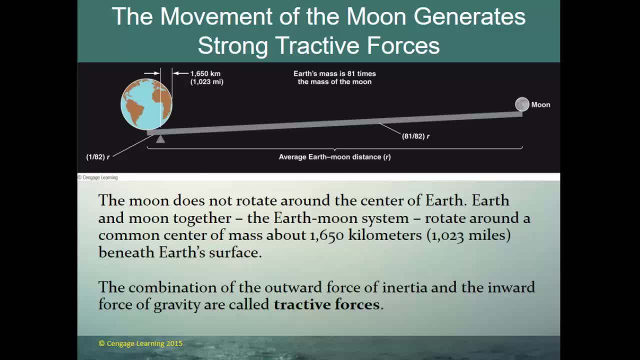 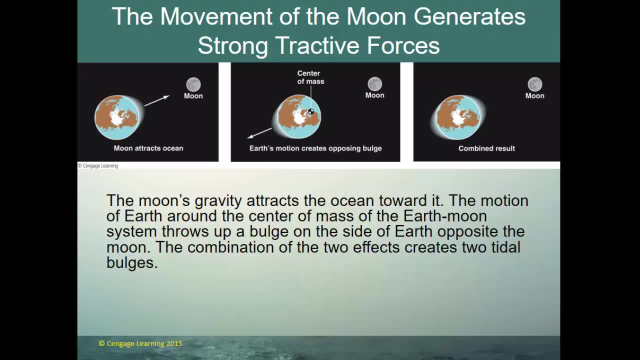 the two revolve around each other- is actually inside the earth's surface, So the moon's gravity attracts the ocean toward it. The motion of the earth around the center of mass of the earth-moon system throws up a bulge on the side of earth opposite of the moon. The combination of the two 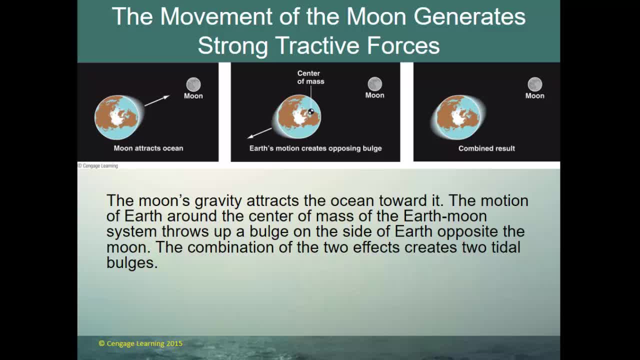 effects, creates two tidal bulges. So in the first illustration you can see where the tractive force of the moon, the gravity of the moon, literally pulls the ocean surface toward it and it creates a bulge on that side of the earth, The earth spinning around that center of mass of the earth-moon. 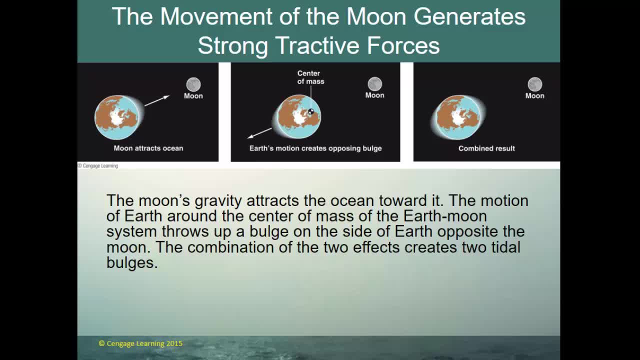 system then forces an opposing bulge on the opposite side of the earth. It's the motion around that center, It's moving around that center and that creates that opposite or that opposing bulge, And the combination is: at any given moment you have a bulge created by the 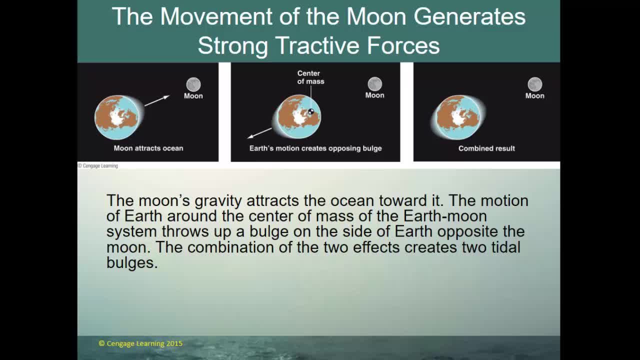 gravity of the moon essentially pointing toward the moon, and on the opposite side of the earth, you have a bulge in the sea surface. This is. this bulge represents the sea surface. Without the moon, the sea surface would be flat around the earth With. 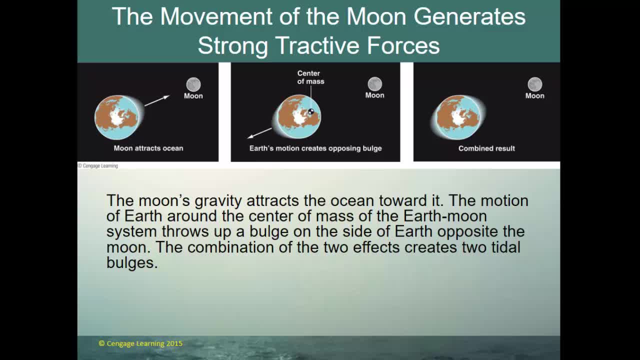 the moon. as you see in the left illustration, there's a bulge toward the moon because of the motion of the earth in the earth-moon system. There's a bulge away from the moon and the combined result is this bulge in the sea surface pointing toward the moon and pointing away from. 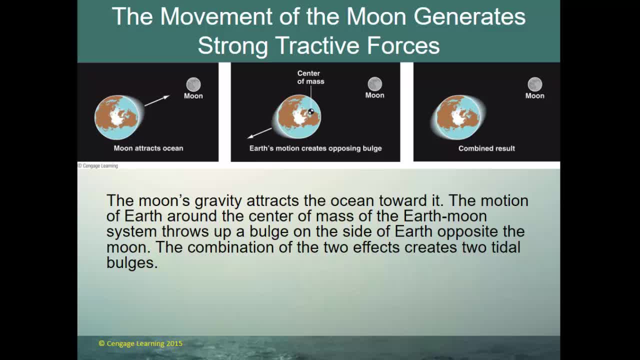 the moon. Those are the high tides. The center of that bulge is the high tide and, as you know, the earth revolves on its axis. It spins on its axis And it's that spinning on its axis that then causes any given beach to go from high tide to low. 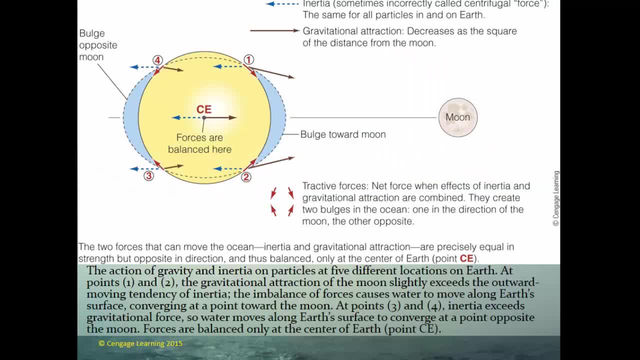 tide back to high tide to low tide. So here's a very detailed explanation of this and you should take a few moments, maybe pause the video and read some of the very specifics about this, where you have different forces at different points on the earth, forces created by inertia forces. 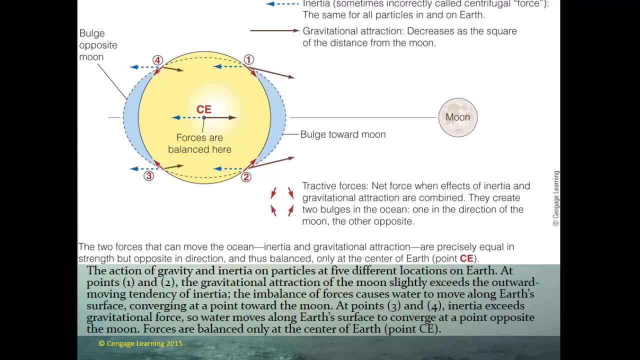 created by gravity, attractive forces, and then how they all sort of balance together, In the end, the two forces that move the ocean, which one is inertia: the inertia on the planet's surface because of our motion around the earth-moon system, and the gravitational attraction of the moon. they are precisely equal in strength, but they are opposite in direction, So that inertia and the gravitational attraction to the moon is the same, Okay, Okay, but just in opposite directions. And so they balance, but they only really balance at the center of the Earth. 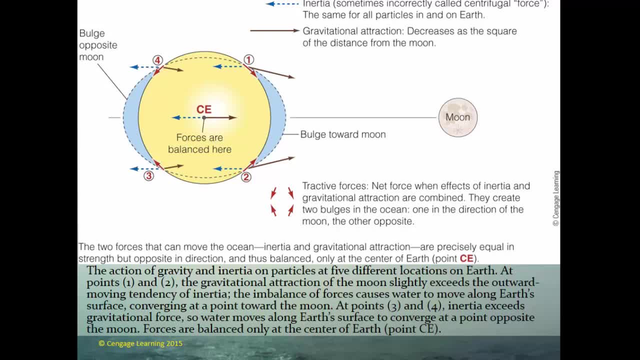 That's the center there, the CE point. The action of gravity and inertia on particles at five different locations on Earth are shown here. So we see it at 1,, 2,, 3,, 4, and then on 5.. 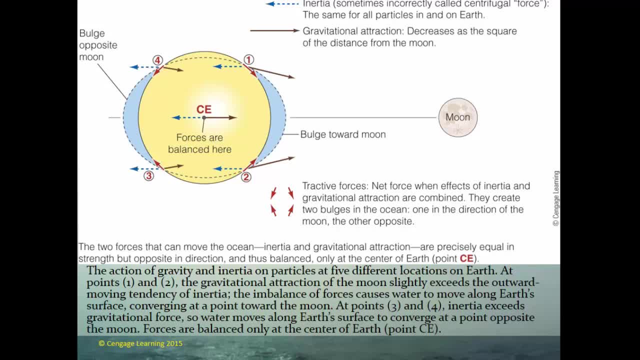 At points 1 and 2,, the gravitational attraction of the Moon slightly exceeds the outward moving tendency of inertia. The imbalance of forces causes water to move along the Earth's surface, converging at a point toward the Moon. At 3 and 4,, inertia exceeds the gravitational force. 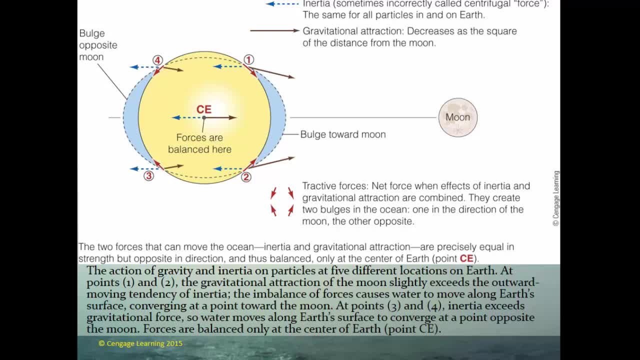 So water moves along the Earth's surface and converges at a point opposite the Moon. So it is that motion of the water along the Earth's surface, because on the side closest to the Moon the gravitational attraction exceeds inertia, and on the side away from the Moon, inertia exceeds gravitational attraction. 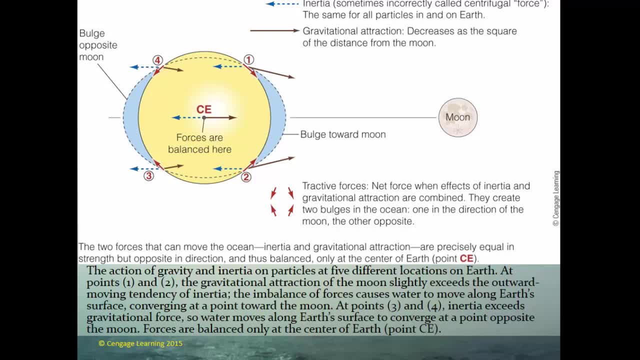 That causes the water to move along the Earth's surface and then bulge up there right in the center, And so again you get a bulge toward the Moon and a bulge opposite the Moon, and the Earth, of course, is revolving underneath that bulge. 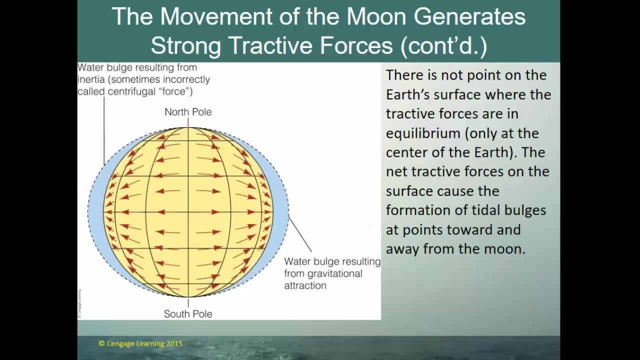 and that is how we go from high tide to low tide. So the movement of the Moon generates those strong tractive forces. The water bulge resulting from inertia is on the backside of the Earth and the water bulge resulting from gravitation. 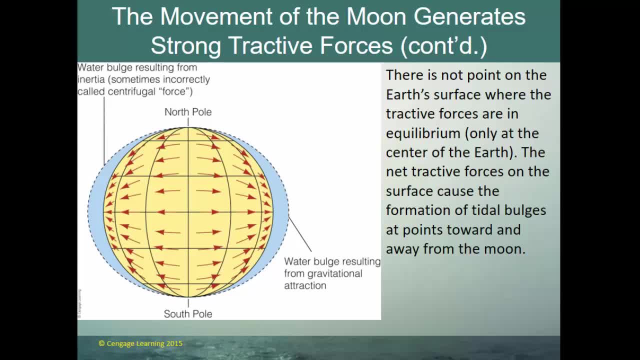 is on the front side of the Earth. There is not a point on the Earth where the tractive forces are in equilibrium, only at the center of the Earth. On the surface of the Earth they're not. So the net tractive forces on the surface causes the water to move toward those bulges. 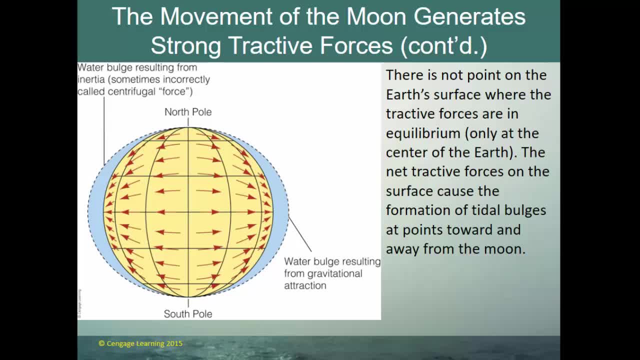 one pointing toward the Moon and one pointing away from the Moon, And again looking at the Earth from the side: North Pole to South Pole, the movement of the planet from the west to the east, the spinning of the Earth counterclockwise. 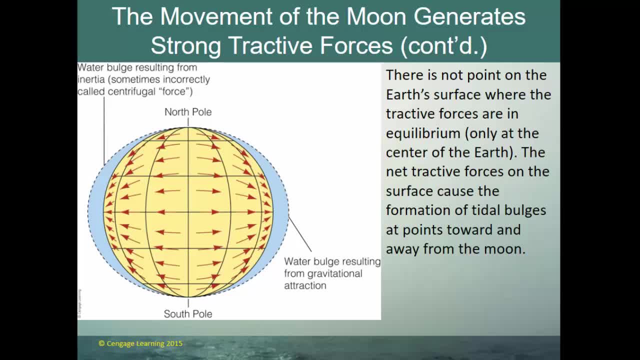 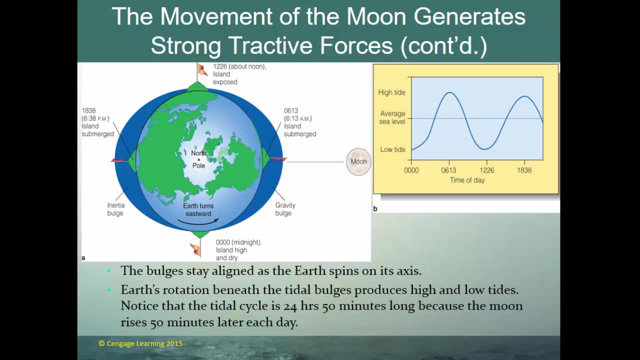 As you look down on top of it. it means that at one point you're going to be under low tide and at another point you're going to be under high tide. The bulges stay aligned. The earth-Moon system doesn't change dramatically over the course of 24 hours. 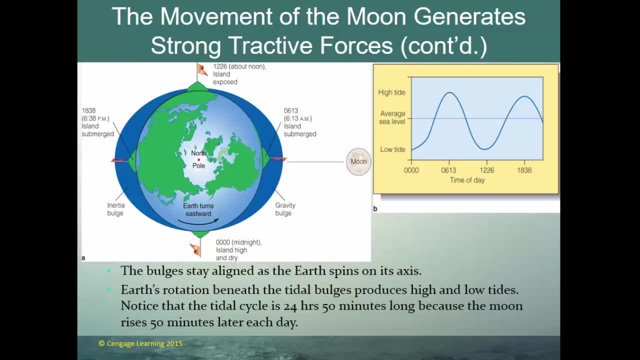 It does. The Moon takes 28 and a half days to get around the Earth. So there is some movement of the Moon along its path around the Earth, but in a given 24-hour period it's nominal, And so that bulge essentially stays put. 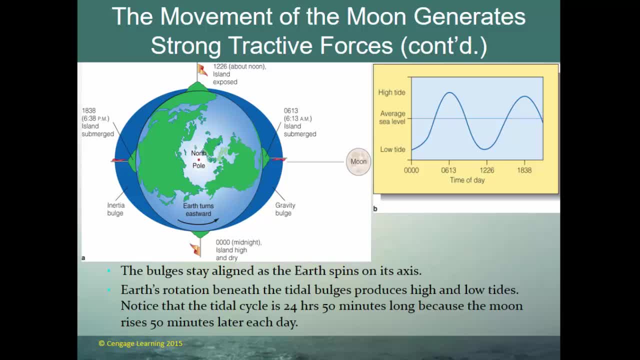 So the bulge stays aligned as the Earth spins on its axis. Earth's rotation beneath the tidal bulge produces high tides and low tides, And we can see, if we look at this, that the tidal cycle is about 24 hours and 50 minutes long. 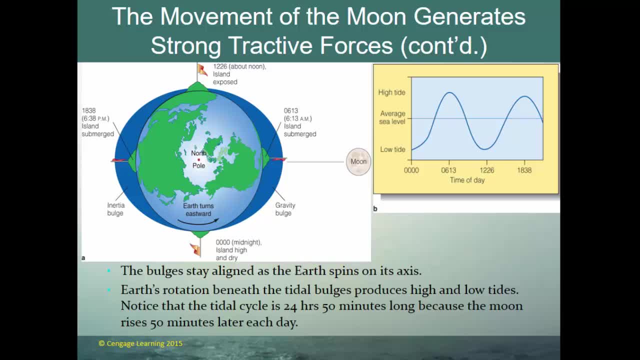 That's because the Moon is going to come up about 50 minutes later each day because of its trip around the Earth every month or so, a little bit less than a month. So it doesn't come up at the same time. It comes up a little bit later. 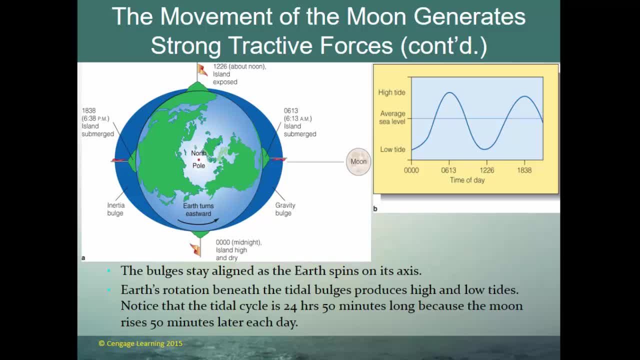 And because of that, the tides change by anywhere between 50 and 40 to maybe 60 minutes a day, depending on which basin you're in. And again, we're looking down on the Earth. The Earth turns eastward, west to east, underneath the tidal bulges. 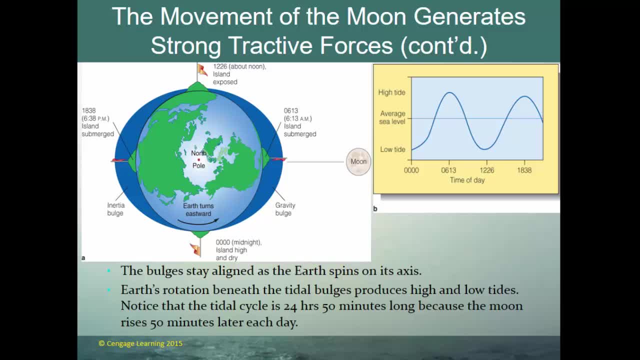 And at one point, at 6.13 in the morning, you have high tide, And then at 12.26, you have low tide, And that's as that island that's showing this illustration spins through. It spins through that tidal bulge. 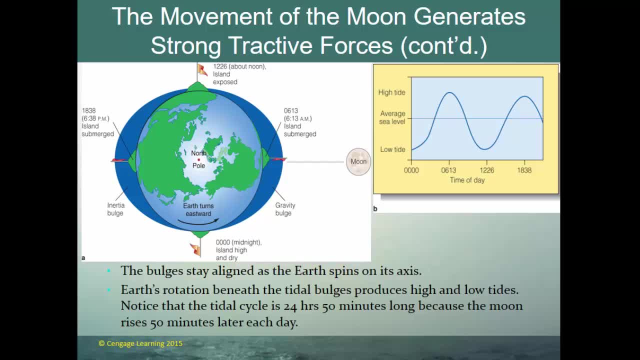 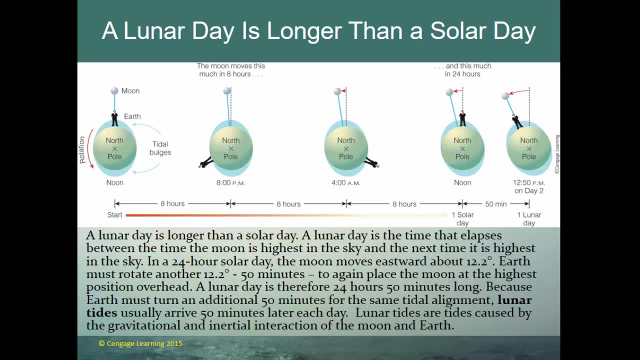 The bulge isn't moving. The bulge is fixed. The Earth itself spins through that bulge. A lunar day is the time that elapses between the time the Moon is highest in the sky and the next time it is highest in the sky. 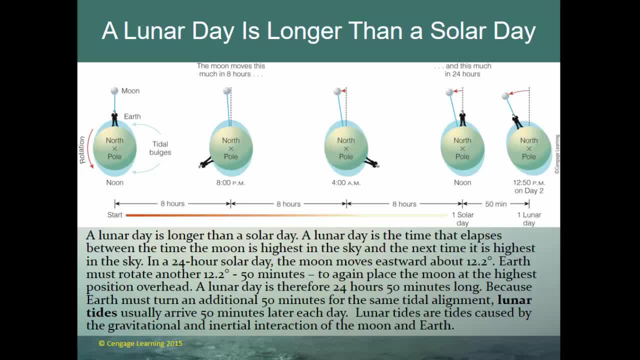 In a 24-hour solar day, the Moon moves eastward by about 12.2 degrees, So Earth must rotate another 12.2 degrees, or about 50 minutes, to again place the Moon at its highest position overhead. So a lunar day is 24 hours and 50 minutes long. 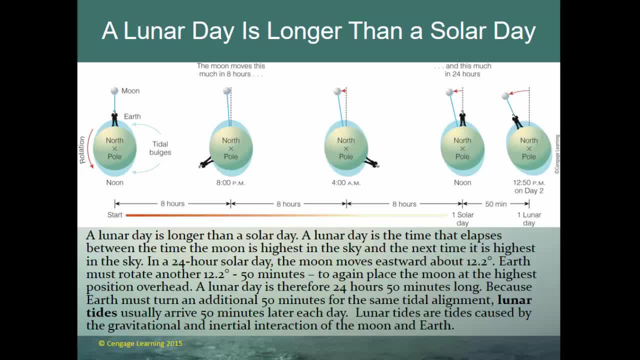 Because Earth must turn an additional 50 minutes for the same tidal alignment. lunar tides usually arrive about 50 minutes later each day. Now again, the dynamic theory tells us that there's other factors involved that change that, So it's not always exactly 50 minutes, but it's about 50 minutes later each day. 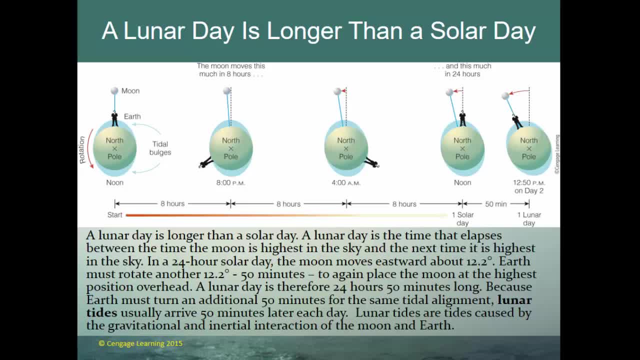 Lunar tides are tides caused by the gravitational and inertial interactions of the Moon and the Earth, And so there's the Moon direction. The Moon is directly overhead at the start, and then, as you go around one solar day, the Moon has moved 12.2 degrees. 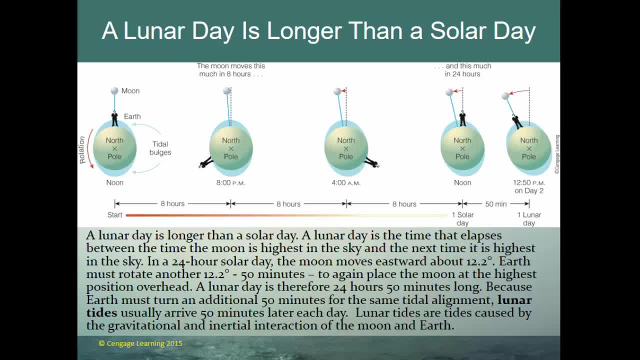 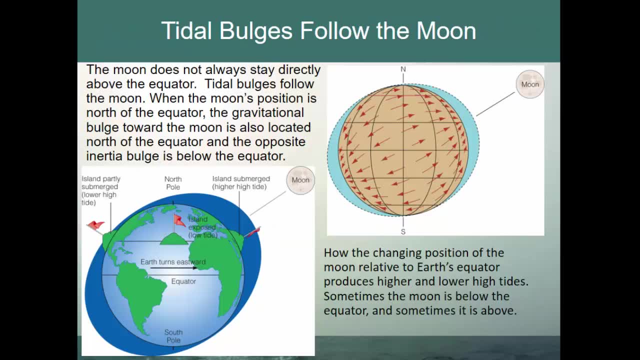 And so you have to travel another 50 minutes to catch up to it. And that's why the tides aren't exactly aligned every day. That's why they're about 50 minutes later each day, So those tidal bulges will follow the Moon. 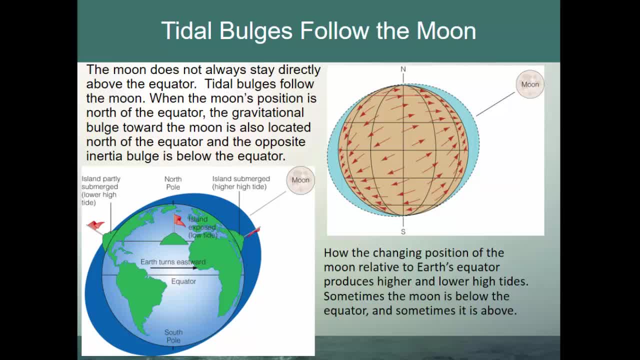 So the tidal bulge will move again with the Moon, And why Our tides are different every day. The Moon does not always stay directly above the equator and tidal bulges follow the Moon. So not only is the Moon moving ahead 12.2 degrees each day, it's not always directly. 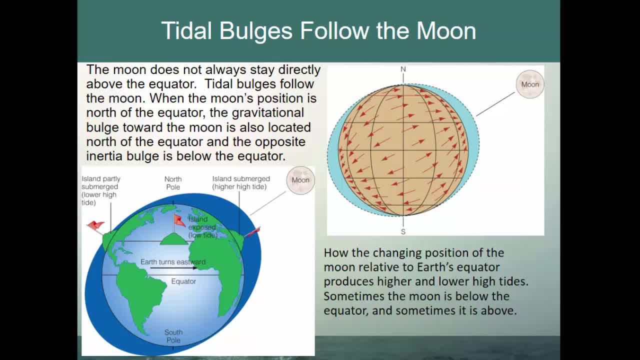 aligned with the equator And because it's not always directly aligned with that equator, that bulge is going to follow the Moon When the Moon's position is north of the equator, the gravitational bulge toward the Moon is also located north of the equator, and the opposite inertial bulge is below the equator. 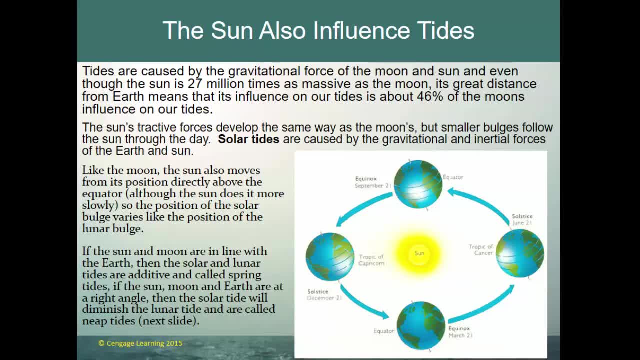 on the opposite side of the Earth. So, yes, the Sun does also influence the tides. Tides are caused by the gravitational force of the Moon and Sun and even though the Sun is 27 million times as massive as the Moon, its great distance from the Earth means that. 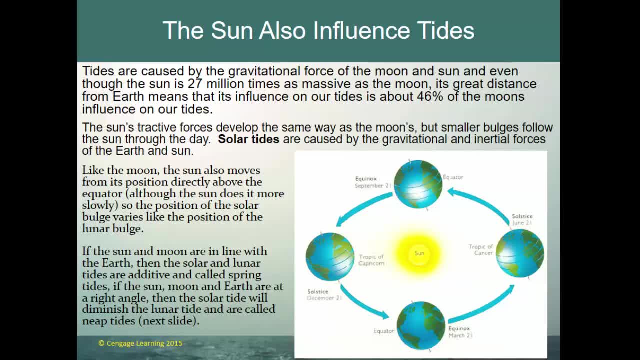 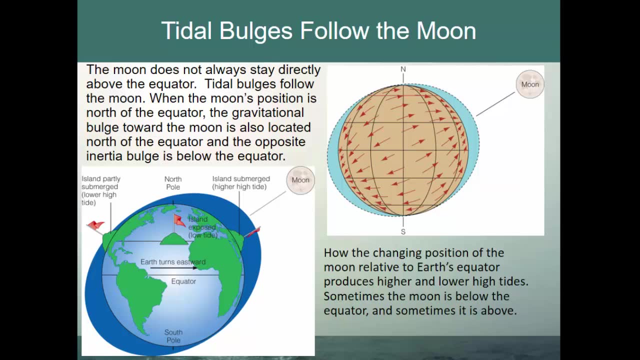 its influence on our tides is only about 46% of the Moon's influence on our tides. The Sun's tractive forces develop the same way. the Moon's, but smaller bulges follow the Sun through the day. In reality, it's not just the one bulge of the Moon. 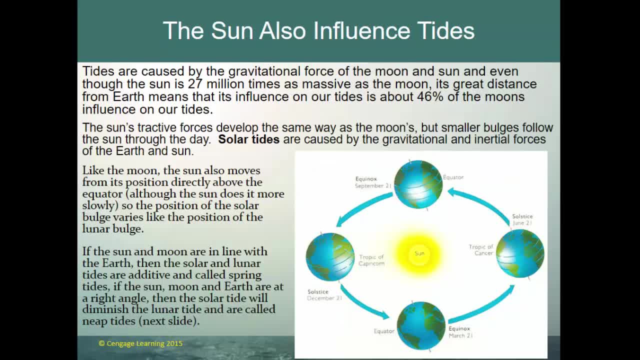 There's going to be one large bulge on either side of the Earth because of the Moon and because of inertia, but there's also going to be a smaller bulge that is created by the Sun. So the Sun's tractive forces develop in the same way as the Moon, but smaller bulges follow. 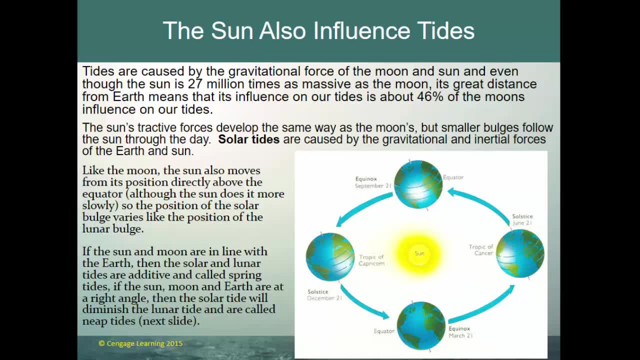 the Sun through the day. Solar tides are caused by the gravitational and inertial forces of the Earth and Sun, very much the same way as with the Moon. Like the Moon, the Sun also moves from its position directly to the Moon. The Moon's position is directly above the equator, although the Sun does it more slowly. 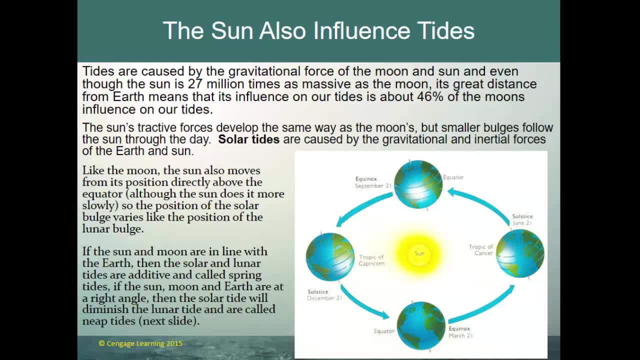 so the position of the solar bulge varies just the same way as the position of the lunar bulge. Again, we're talking about that north and south of the equator. At the equinox, or the beginning of fall, the beginning of spring, the Sun is directly. 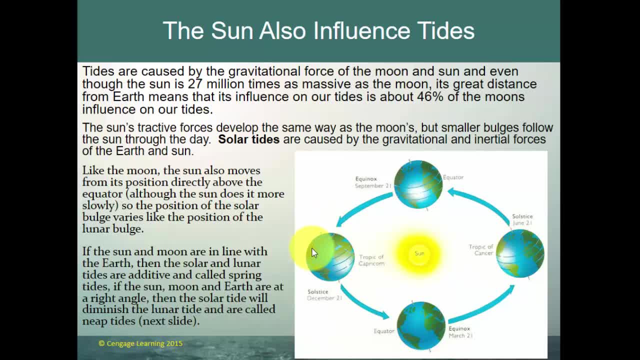 over the equator and that's where the bulge would be. But when we go into the northern hemisphere winter and we're tilted away from the Sun, the bulge is down here over the Tropic of Capricorn, So that's where the bulge will be. 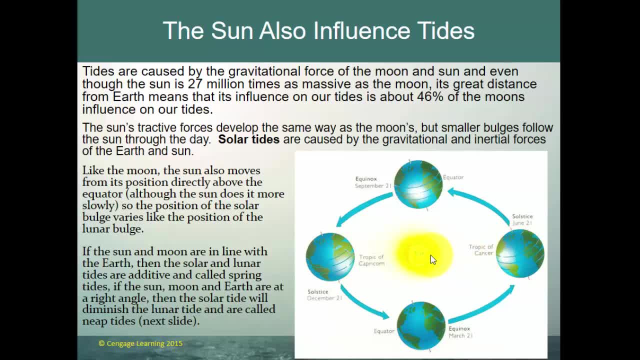 And same thing when we go into our solstice in June. the Sun is directly over the Tropic of Cancer and that's where the bulge would be. If the Sun and the Moon are in line with the Earth, then the solar and lunar tides are. 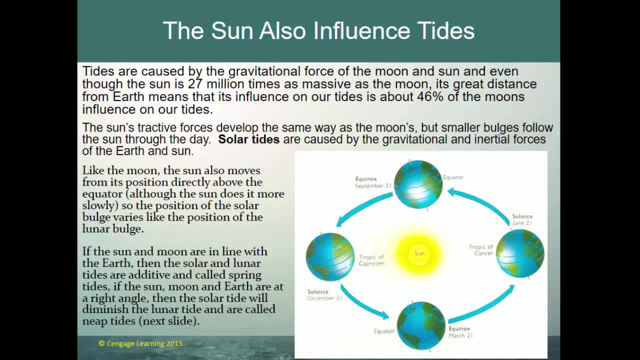 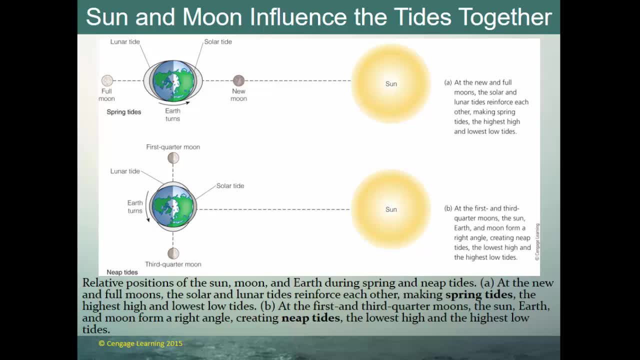 additive called spring tides. If the Moon and Earth are at a right angle, then the solar tides will diminish and the lunar tides are called neap tides. So this is a reference to the solar tides themselves. So I'll go back and it says: if the Sun and the Moon are in line, then the solar and lunar 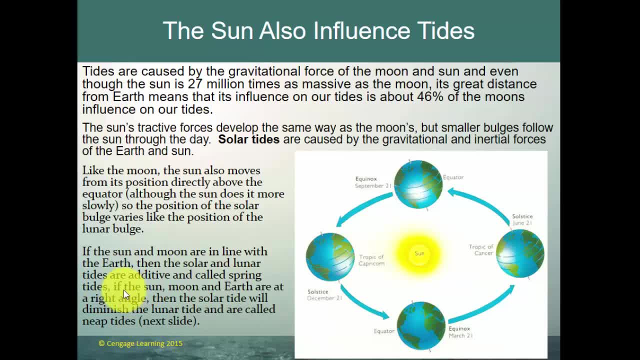 tides are additive and they're called neap tides. If the Sun and the Moon are in line, then the solar and lunar tides are called spring tides, And if the Earth is at a right angle with the Moon, then the solar tides will diminish. 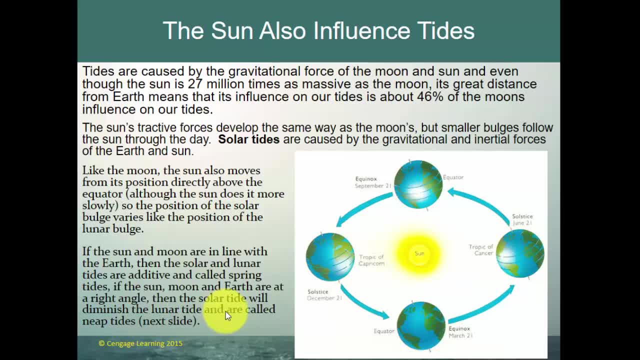 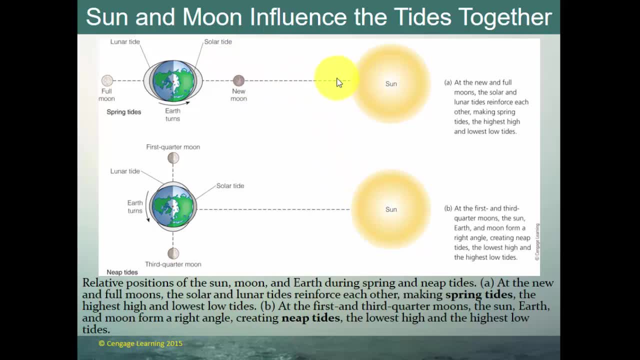 The solar tide will diminish and the lunar tide is called a neap tide, So that's what this looks like. So when you have a new Moon again. so here's the Sun shining on the Moon, shining on this side of the Moon. 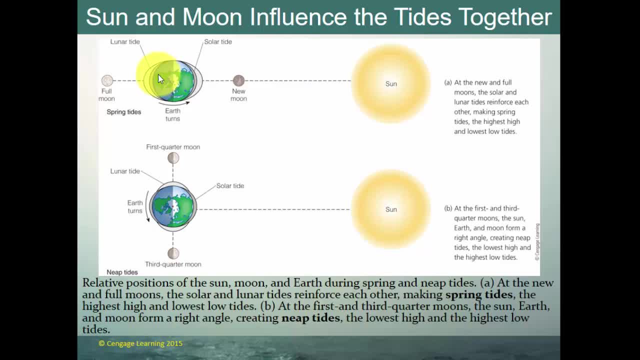 So what we see at night is dark. That's a new Moon, And here's the Sun shining on the Moon, and, other than some type of an eclipse, the full half of the Moon is going to be illuminated, So that's going to be negative. 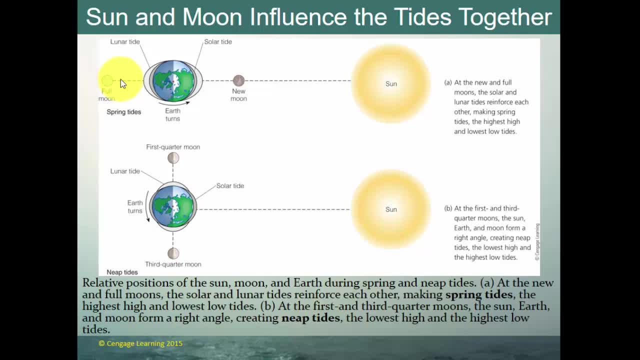 So that's going to be a full Moon, And so when you have the Moon on the opposite side, it's going to pull this bulge further out, And you have the Moon on this side, it's going to pull this bulge further out. 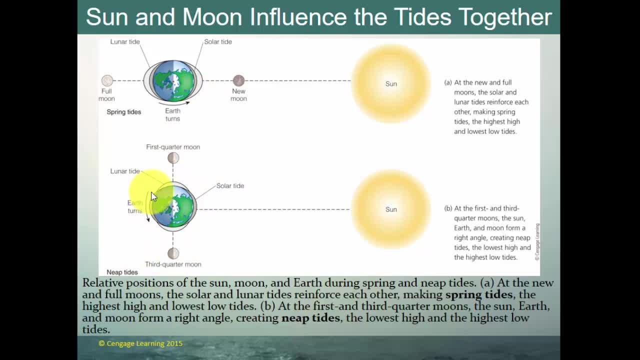 When the Moon is at that right angle, then the lunar bulge is here, and the lunar bulge is here and the solar bulge is here, And so you've lessened the tides In this situation: you're adding the solar and the lunar. 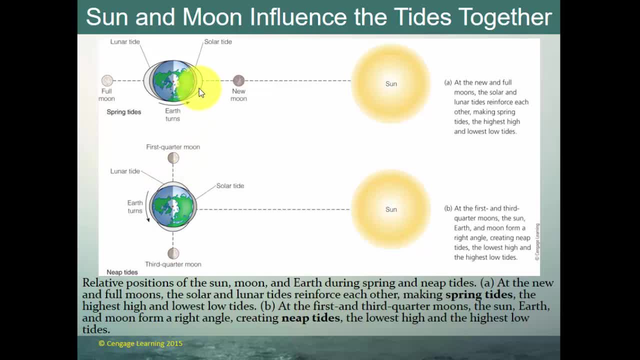 And you're adding the solar and the lunar And here you're subtracting them, So your high tides are going to be higher during your spring tide, the additive tides And your low tides are going to be lower. And then here, your high tides are not going to be quite as high, but your low tides are. 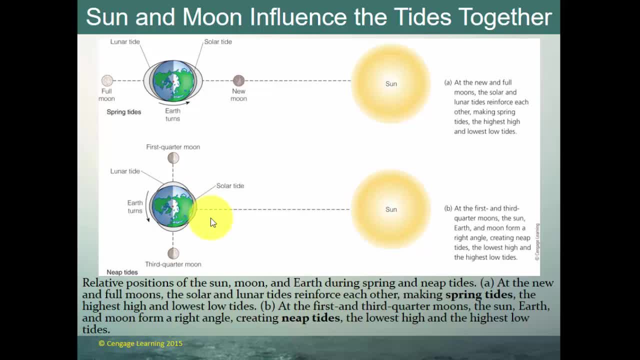 going to be a little bit higher. There's going to be a little bit higher low tide as well. So bottom line is: at the new and full Moon, the solar and the lunar tides reinforce each other, making spring tides the highest tides and lowest tides. 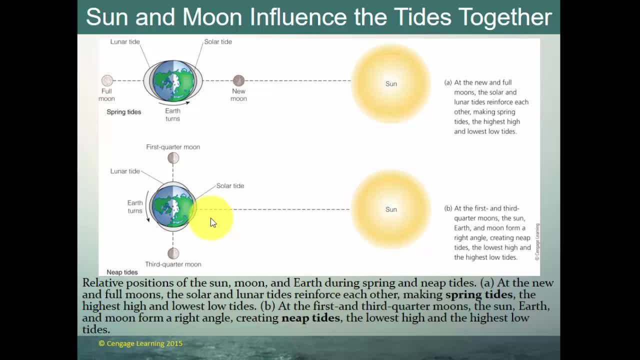 At the first and third quarters, the Sun and the Earth And Moon form a right angle, creating neap tides, the lowest highs and the highest lows. So it's the lowest highs and the highest lows. Relative position of the Sun, Moon and Earth during spring and neap tides. 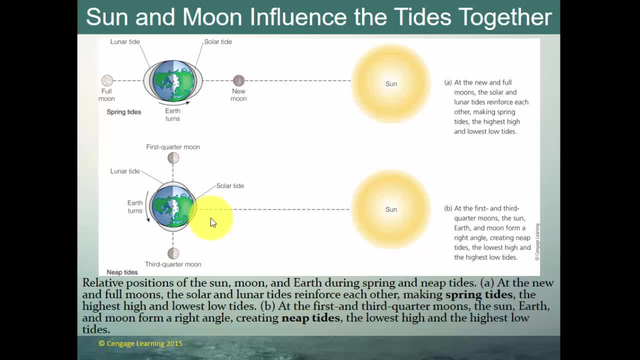 You can see that here All the new and full Moons, or I should say, at the new and full Moons, the solar and lunar tides reinforce each other, making those spring tides the highest high and the lowest low. 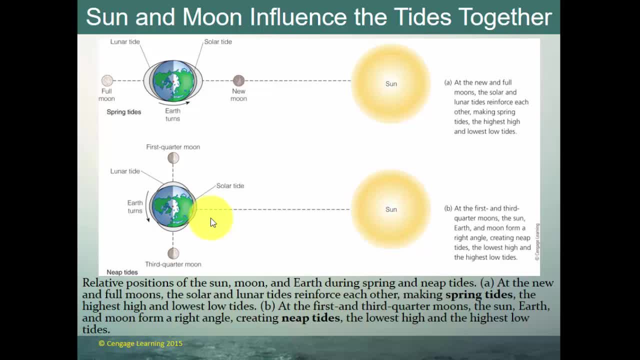 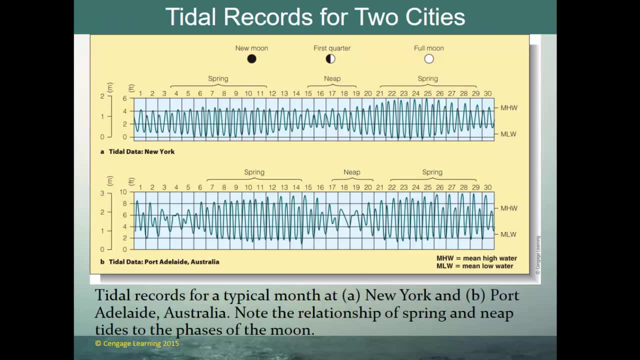 At the first and third quarter, the Moon, the Sun and the Earth form a right angle, creating neap tides: the lowest high and the highest low tide. Here you can see the tidal record for two cities, New York City and Port Adelaide. 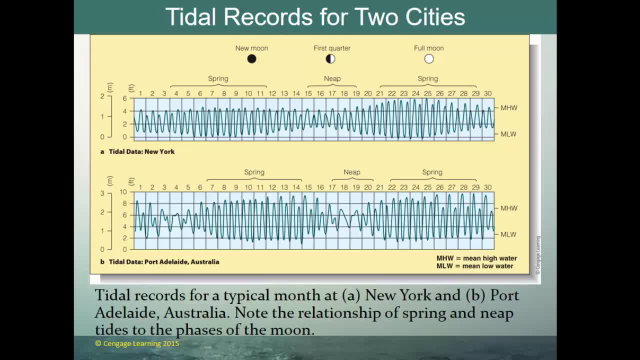 Australia and the impact of the phases of the Moon. Remember, at the new Moon and the full Moon the Sun and the Moon are lined up and that creates additive tides. So the tides are going to be higher And then at the quarter you are going to have lower high tides but your actual low 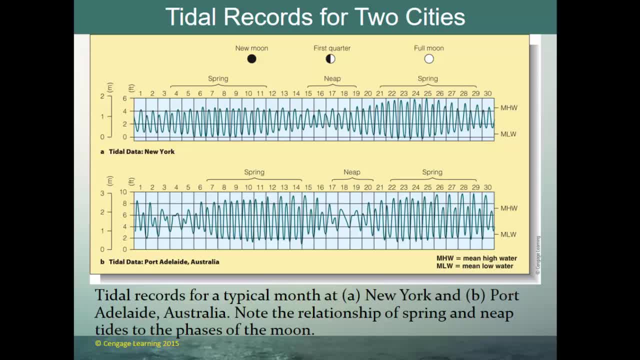 tides will be higher. So there's definite changes between the spring tide and the neap tide And they all follow the phase of the Moon. And again, the Moon is not always in the exact same position over the Earth. every day It changes by about 50 minutes. 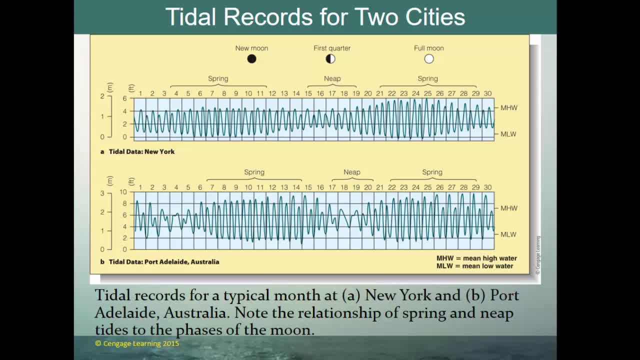 So this all fluctuates with great curiosity, And then you have other factors that determine when high tides and low tides are going to occur. So it's never all exactly the same one day to the next, one month to the next, or one. 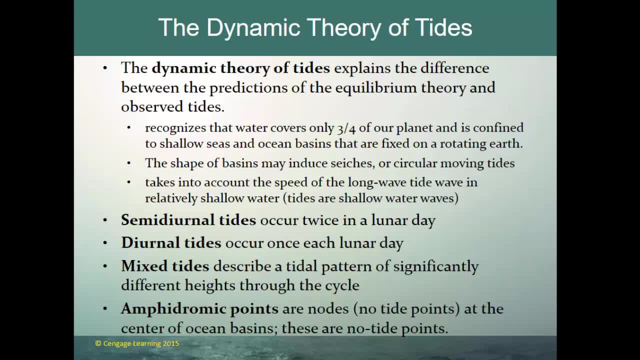 year to the next. The dynamic theory of tides explains the difference between the predictions of the equilibrium theory and the observed tide. So the equilibrium theory explains the difference between the predictions of the equilibrium tides and the observed tides. So the equilibrium theory would predict one thing. 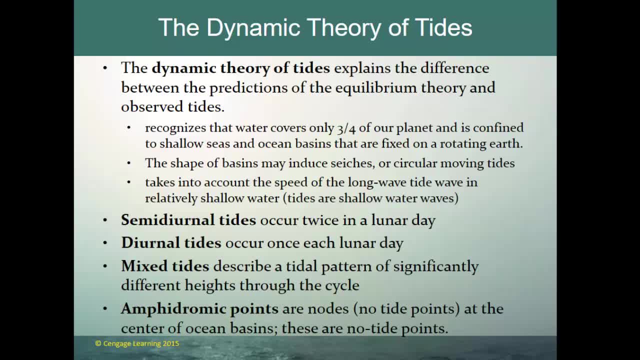 The actual observed tides are something different And we use the dynamic theory to explain the difference. It recognizes that water covers only three quarters of the planet and is confined to shallow seas and ocean basins that are fixed on the rotating Earth, And it also understands the shape of those basins may induce different types of tidal. 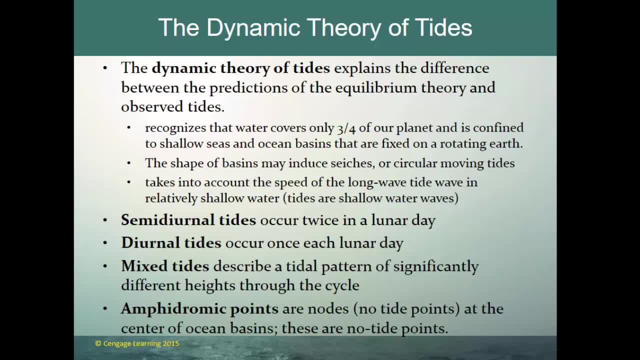 movements, including seashes, water sloshing back and forth or circular moving tides. It also takes into account the speed of the long wave tide. And it also takes into account the speed of the long wave tide in relatively shallow waters. 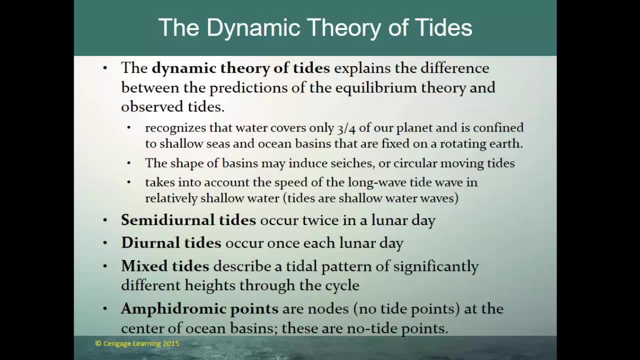 Tides are always shallow water waves, They always feel the bottom. So we have different types of tides, three basic different types of tides: semi-diurnal, diurnal and mixed tides. And so the word diurnal means daily. 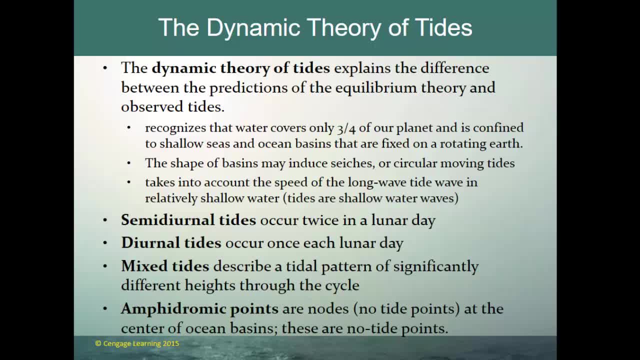 You probably are familiar with the idea of something being nocturnal, something that occurs at night. We oftentimes say that cats are nocturnal animals. They do most of their activity at nighttime. Well, diurnal means daily, Diurnal means twice a day or half the day, so twice a day. 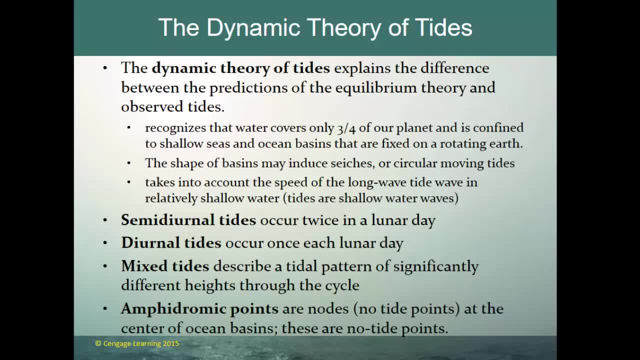 Diurnal means once a day, And then there's mixed tides, So semi-diurnal tides occur twice in a lunar day, That's in a lunar day. Diurnal tides occur once each lunar day, And then mixed tides describe a tidal pattern with significantly different highs and lows. 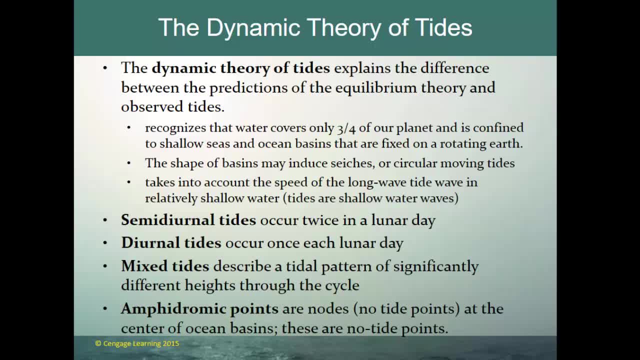 through a cycle. Now, within all basins there's an amphidromic point or the amphidromic points, which are nodes. So the amphidromic point or node is a no-tide point where the water does not change. 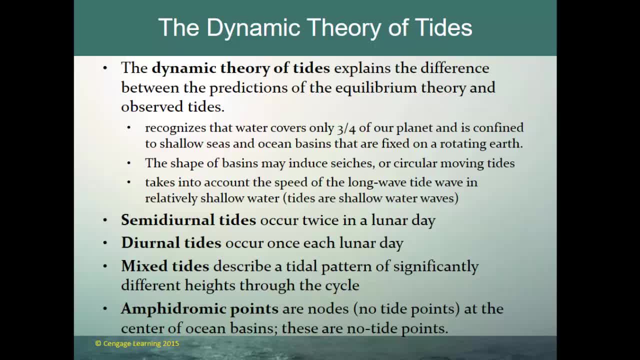 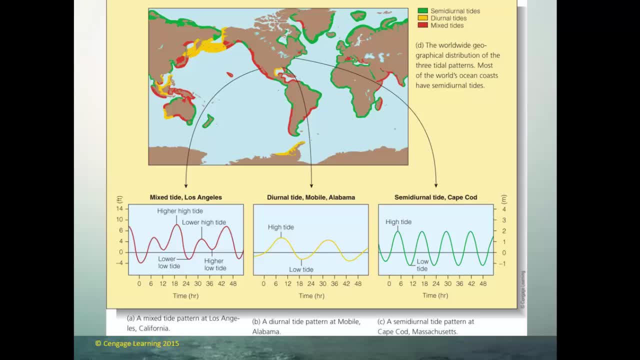 At the center of ocean basins. this is where the water level does not change. So here is an illustration globally, where you have mixed tides, like Los Angeles, where you have sometimes high, sometimes low, sometimes higher lows and sometimes lower lows. 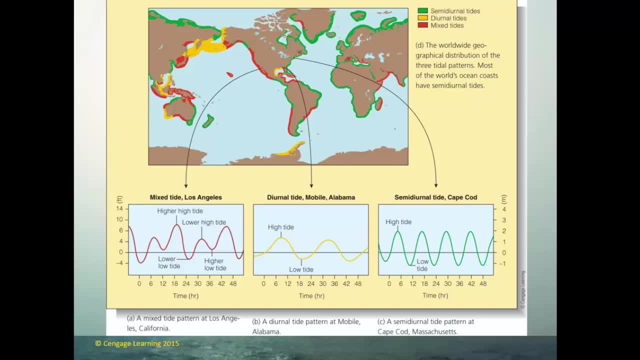 Diurnal tides, meaning one high and one low, and that typically happens in the Gulf Basin because the water kind of sloshes back and forth- And then what we have along the East Coast and what you can see along a big chunk of 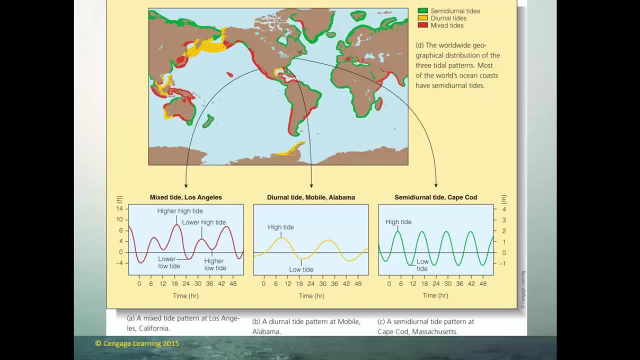 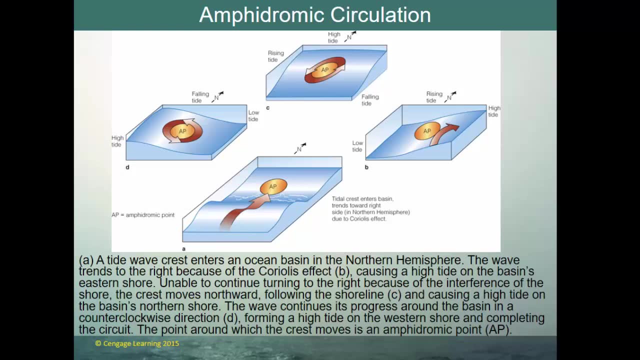 the world's coastlines, the semi-diurnal high, The semi-diurnal high, where you have two high tides and two low tides in any lunar day. So here's the amphidromic circulation: A tide, wave, crest enters an ocean basin in the Northern Hemisphere. 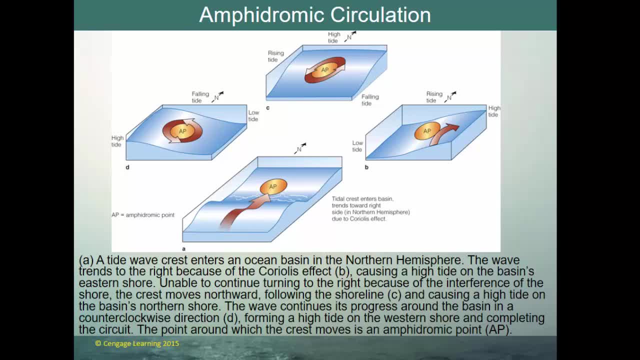 That is what's happening at A. So a tide wave moves into an ocean basin in the Northern Hemisphere. The wave trends, The wave moves. The wave tends to the right because of Coriolis effect, causing the high tide on the basin's. 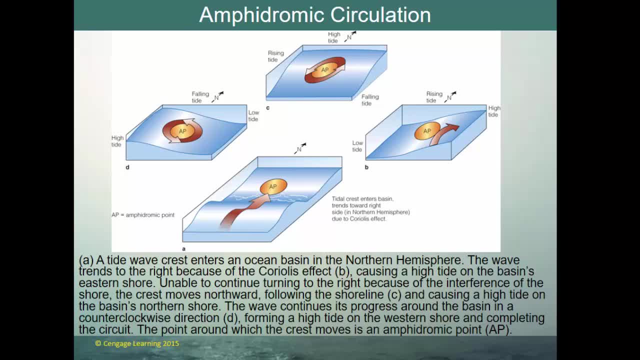 eastern shore, Unable to continue to the right because of the interference of the shore, the crest then gets deflected northward or to the north and follows the shoreline. That causes a high tide on the basin's northern shore. next then, the wave continues its progress. 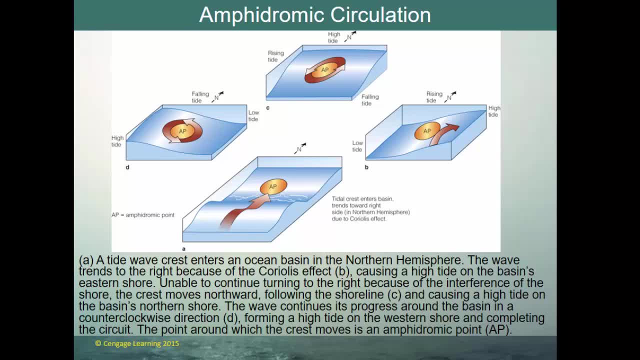 around the basin in a counterclockwise rotation, forming a high tide on the western shore. third, and then completing the circuit, The point at which the crest moves, that point at the center at which the crest moves is the amphidromic point or the AP. 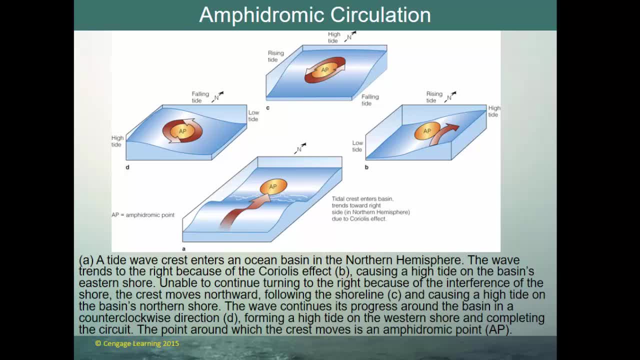 And that is a point where the water level doesn't change. The tide rotates around that point And it may be counterintuitive that it rotates counterclockwise because it's being forced to the right, or clockwise in the Northern Hemisphere, but it's not forced at a 90 degree. 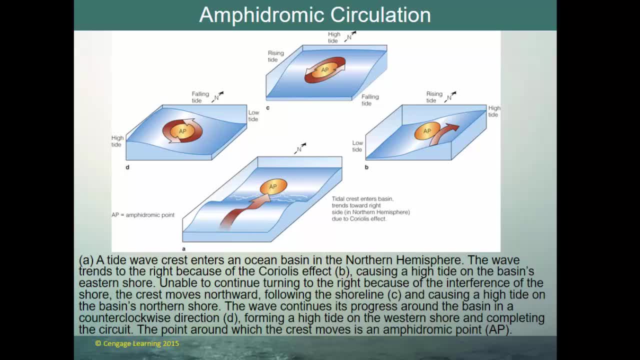 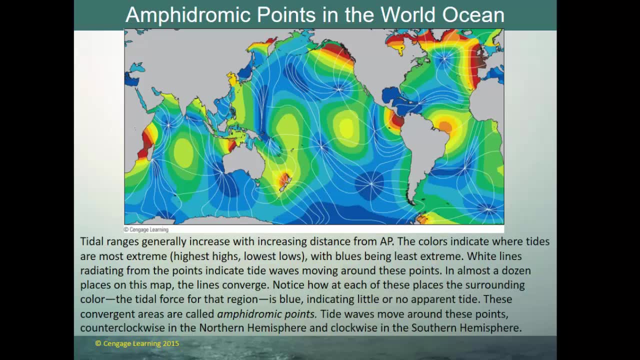 angle. It's forced at about a 45 degree angle, So that wave hits the coast at an angle And it is deflected northward And that's why it wraps around the basin counterclockwise. So these are the amphidromic points in all of the world's oceans. 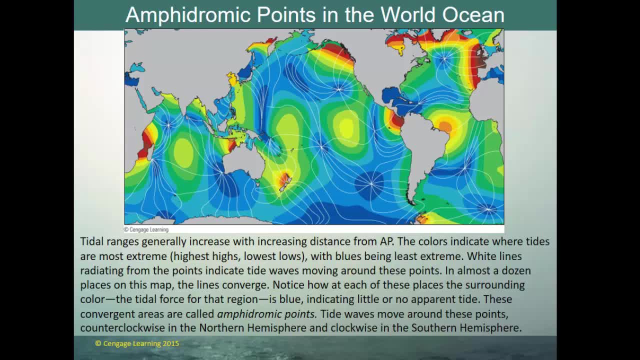 And you can see the North Atlantic has one, You have one sort of in the Caribbean, You have one down in the southern parts of the South Atlantic and the Southern Pacific. There's a couple actually in the Pacific Ocean And each of these amphidromic points are points at which tides rotate around the basin. 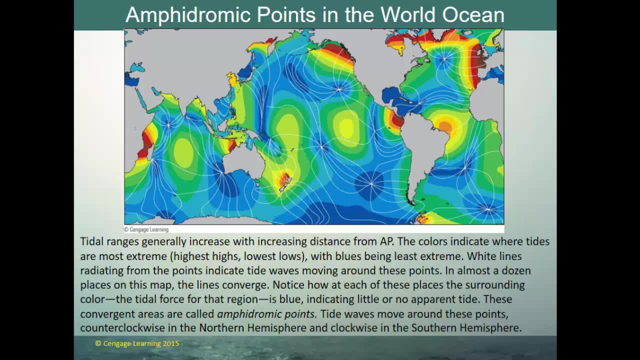 So tidal ranges generally increasing with increasing distance from the AP. So the further you get away from the amphidromic point, the more you're going to have a range of tides. The colors indicate where tides are most extreme, the highest highs and the lowest lows, with. 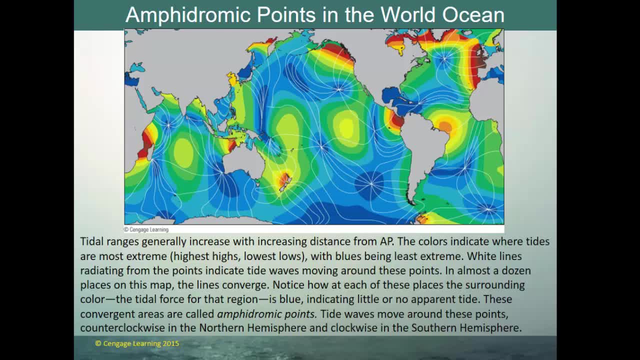 blues being the least extreme and then the reds being the most extreme, And we do have areas where we have extreme high and low tides. They're great distances from the APs, White lines radiating from the AP And the reds being the most extreme. 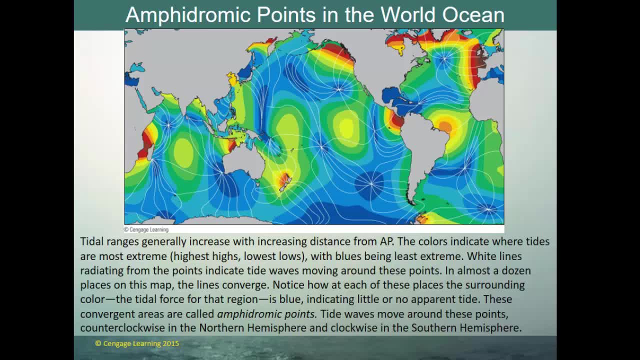 indicate tide waves moving around these points. So there's almost a dozen places on the map where the lines converge. Those are going to be your APs. Notice how, at each of these places, the surrounding color, the tidal force in that region, is blue. 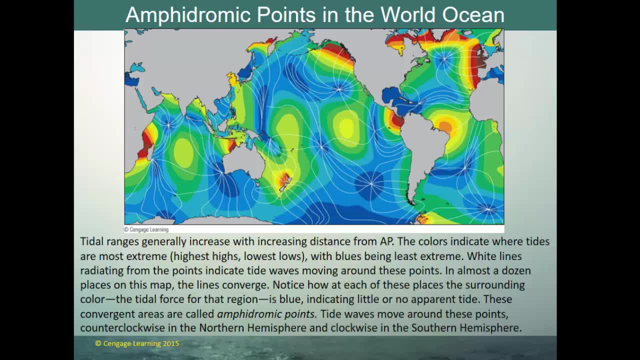 indicating there's little or no apparent tide. That's that amphidromic node, that point in which there's no tide, the no-tide point. These converging areas are called the amphidromic points. Tide waves move around these points clockwise. in the northern hemisphere. 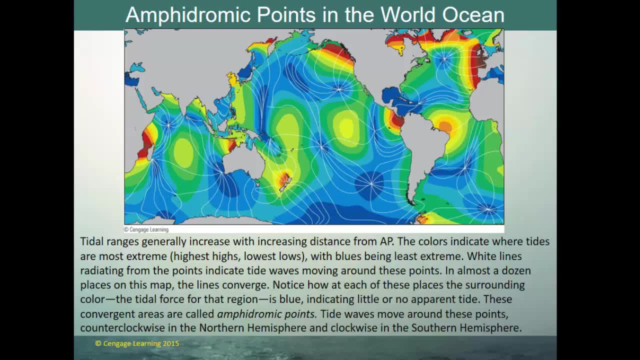 and counterclockwise in the northern hemisphere and then clockwise in the southern hemisphere. I should point out, this whole motion around these very specific points is why tides are so different in so many different parts of the world, And these points change over geologic time. 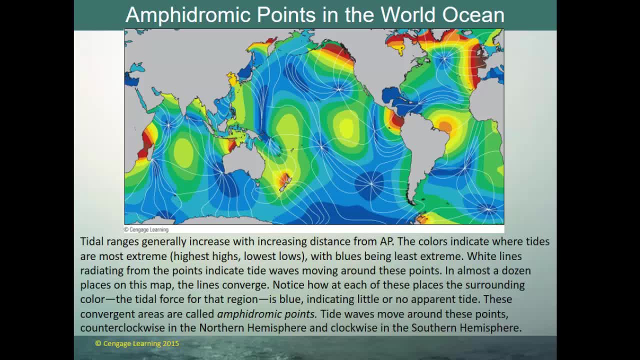 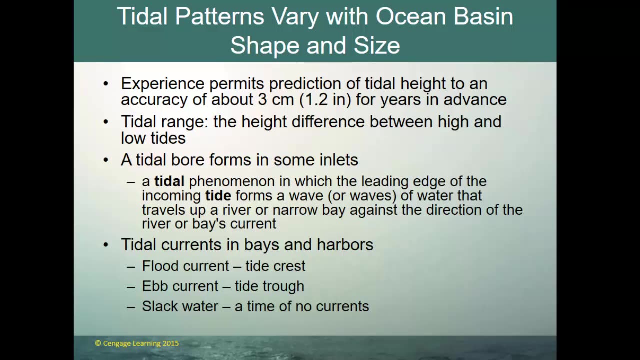 as our continents and ocean basins slowly change their shape, whether increasing or decreasing in size or changing their shape in general- These no-tide points will change as well. It's just an extremely slow process, So tidal patterns vary with ocean basin shape and size. 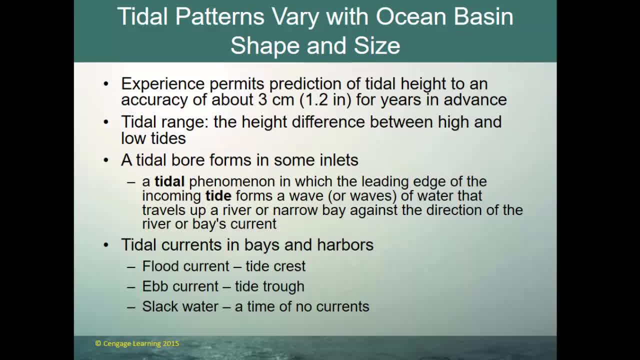 Experience certainly allows the prediction of tide heights to an accuracy of about an inch inch and two-tenths for literally years in advance. The tidal range is the height difference between high tides and low tides. Now in some inlets or other. 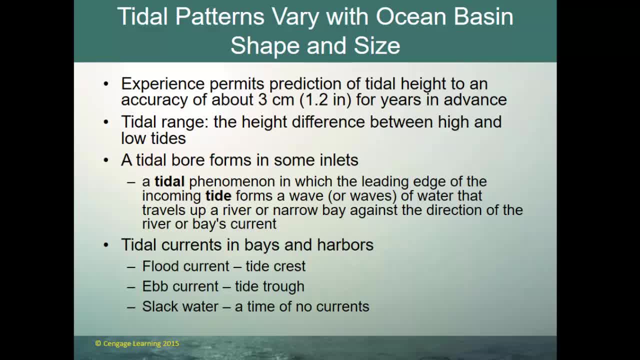 enclosed basins. essentially, you get a tidal phenomenon in which the leading edge of the incoming tide literally forms a wave. So the tide is moving in against water, It's coming in an inlet, And so where a tidal bore forms, is where the leading edge of the incoming tide. 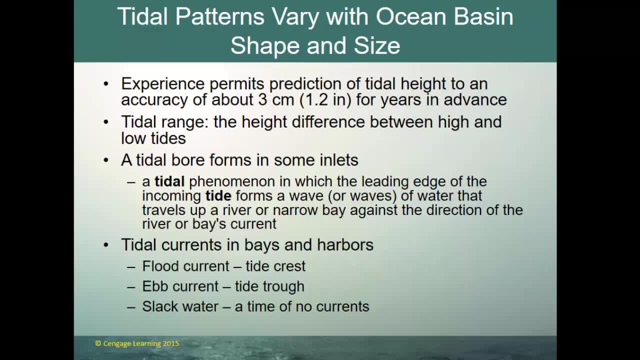 literally forms a wave, or, in some cases, multiple waves of water that travel up the river or up narrow bays, and they literally travel against the direction of the river or bay's current. Now we also have unique tides that occur in bays and in harbors. 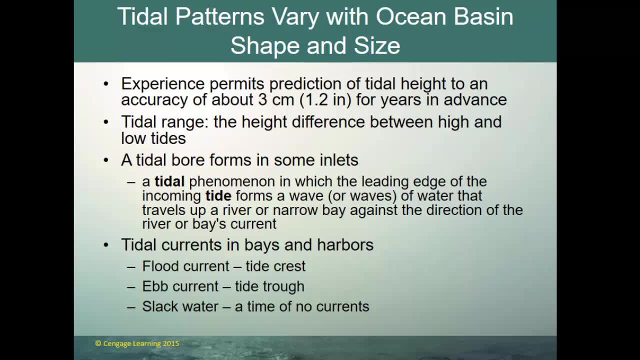 You have the flood current, which is when the tide is crested. You have what's known as ebb current, which is when it's at its lowest point, And then slack water is the time when there's no water moving in or out of the bay or harbor. 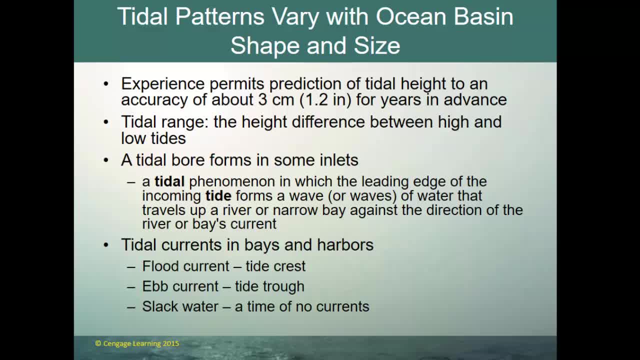 So when the highest amount of water is in the bay or harbor, you're at a flood current. When the lowest amount, you're at an ebb current And when you're in between, it's called slack water. So here's some. 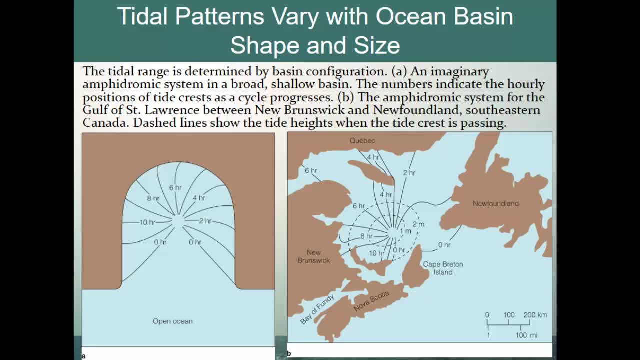 interesting ocean basins and some interesting tidal shapes. So if you look at the open ocean in the left with an AP right in the middle of the basin, the water moves into the basin, deflected to the right, strikes the coastline on the east side. 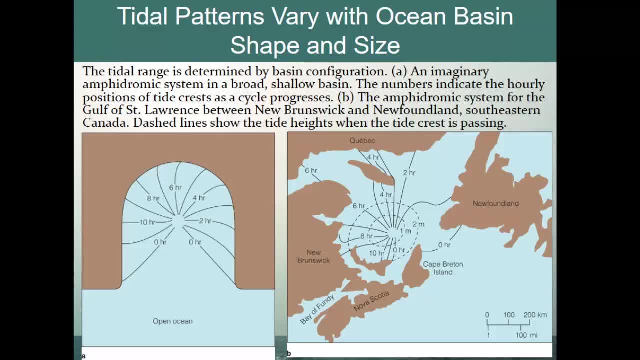 and then just travels around that coastline, taking 10, 12 hours to occur. You have a similar situation that occurs up in the Canadian Maritime Provinces, but the islands and the shapes of the coastline deflect and change those tides. 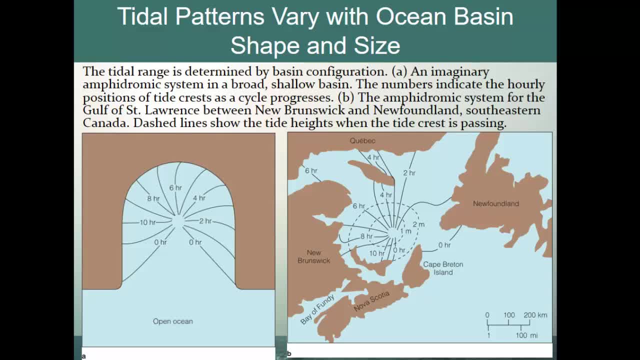 And so it's not exactly the equilibrium theory. Here you have to take into account the dynamic theory. So this tidal range is determined by the basin configuration. So the imaginary AP system in a broad shallow basin. the numbers indicate the hourly position of the tide crest as the cycle progresses. 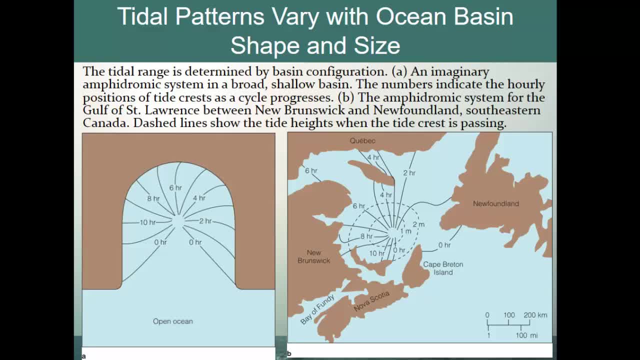 The AP system for the Gulf of St Lawrence again, which is the Canadian Maritimes between New Brunswick and Newfoundland, southeastern Canada. the dashed line shows the tide heights when the tide is passing, So you get some pretty significant tide heights moving through this basin. 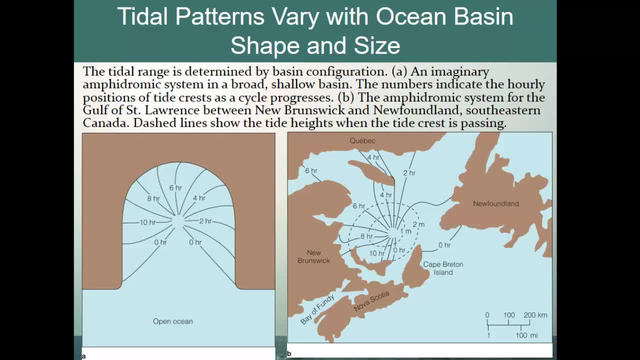 because it's enclosed and you have different, unusual and unique shapes. And if you look at the bottom left-hand corner, the Bay of Fundy is a tidal bay that has one of the largest tidal ranges in the world, where there's literally 20 or 30 feet of tidal range. that occurs 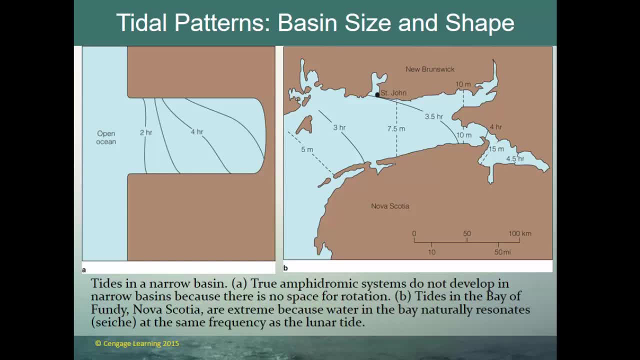 So in a narrow basin, like you see in that A, there's no AP system. There's really no AP because it's so narrow so there's no space for rotation. So as we see, like in the Bay of Fundy, the water just comes straight in and then goes straight back out. 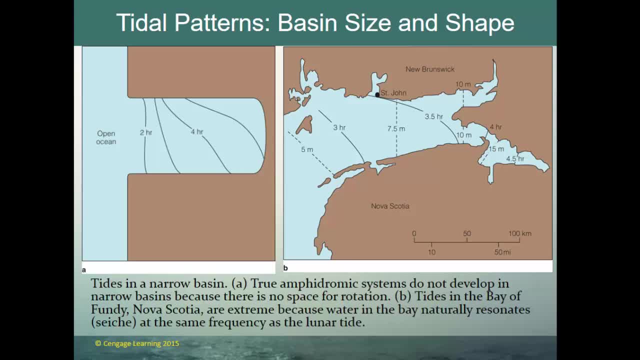 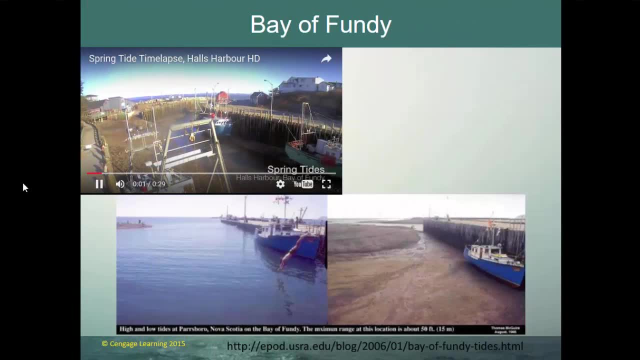 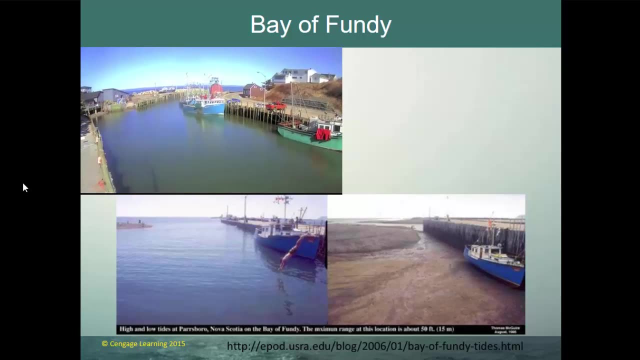 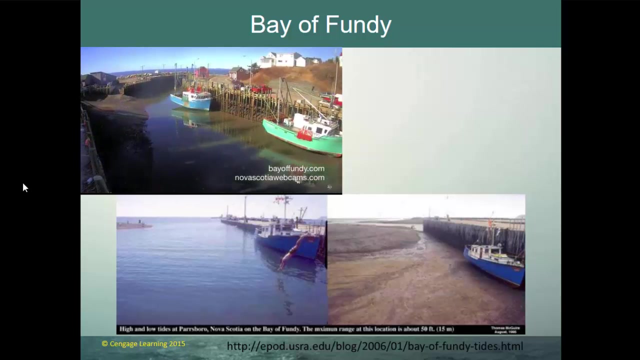 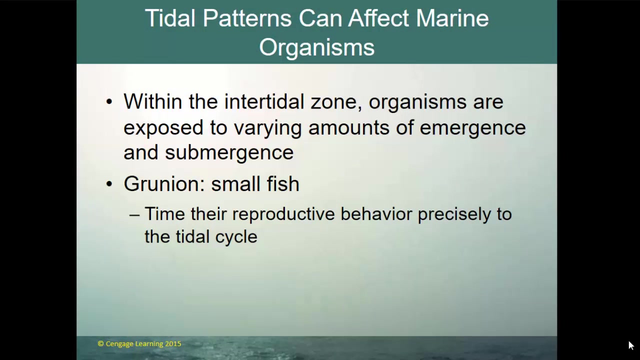 And it creates essentially a sea where water rushes up and water rushes down And you can see there's like a 15-meter tidal range in the Bay of Fundy. Now we are going to talk about tidal patterns and how they affect marine organisms. 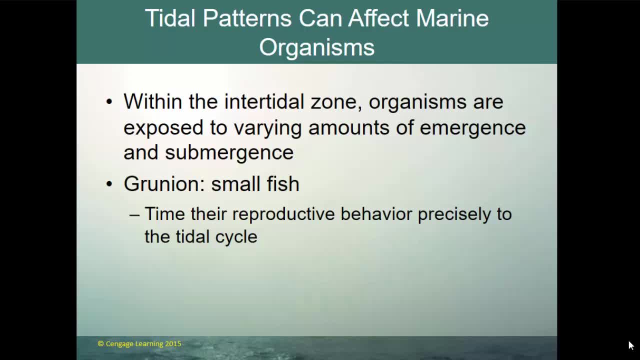 And within that inner tidal zone, the zone where the tide goes from low to high tide organisms are exposed to varying amounts of emergence and submergence under the water, And so it has a dramatic effect on the type of organisms that can live there. 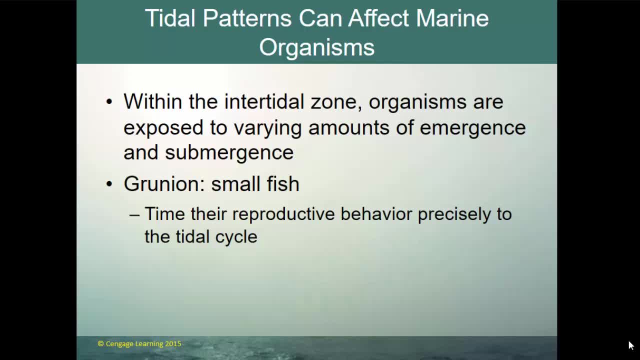 like the grunion, which is a small fish, They time their reproductive behavior to precisely coincide with the tidal cycle, so they can get up on shore during very, very low tide and lay their eggs right on shore. And if you ever heard the grunion run in California. 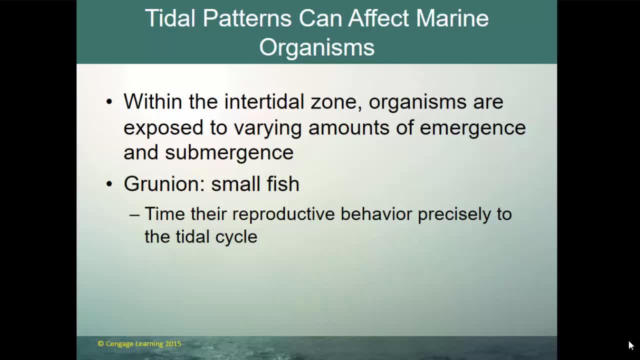 these fish flop up on shore right at the edge of the water and literally lay their eggs in the sand And then, as the water rushes back up, so they do it at the lowest tide of the season and the water comes back up, it covers the fish eggs in water and then the baby fish hatch out of those eggs when it's underwater and swim off. 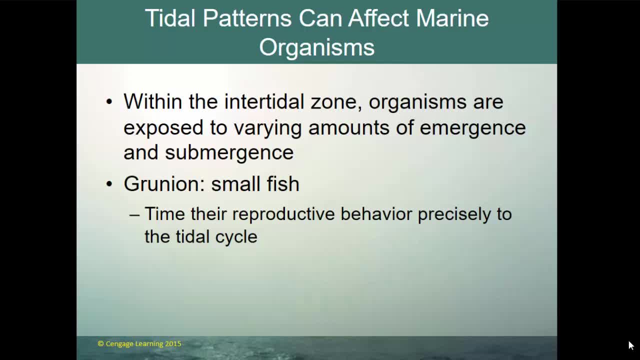 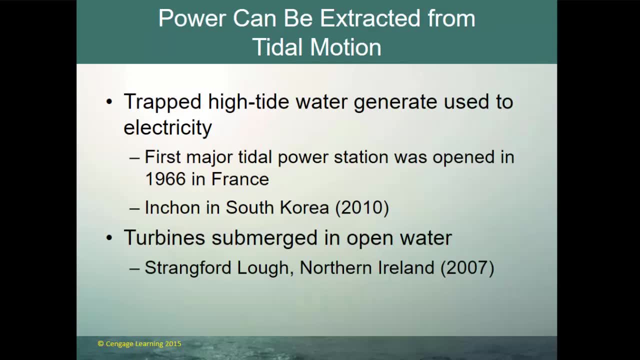 And that's the grunion run. And these grunion can time the length of their eggs precisely to the lowest low tide of the season. And of course, there are lots of other creatures that you find in what are known as tide pools, pools of water that are left behind as tides go up and down. 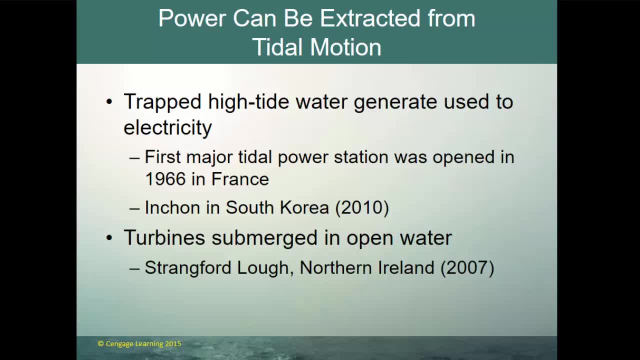 And it's always fun to wade through the tide pools and find the urchins and the crabs and the different things- you know the sea enemy, maybe even sea cucumbers, that you can find in tidal pools. So we also want to talk a little bit about the power that can be extracted from tidal motion trapped. 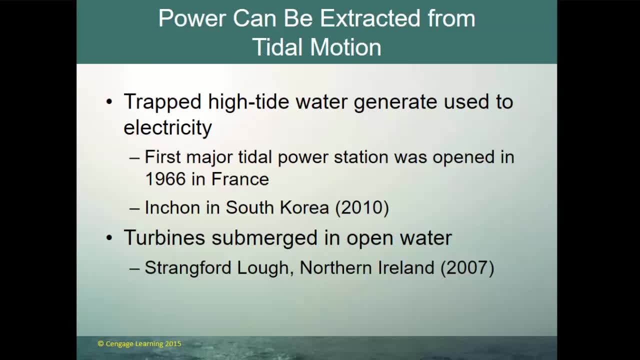 High tide water can be generated to use electricity. So the tide comes in, So it goes up, it's going up slope, it's being pushed up slope, And so the force of gravity is going to pull it back down as the tide goes low, and we can use that force of gravity and water to create electricity. 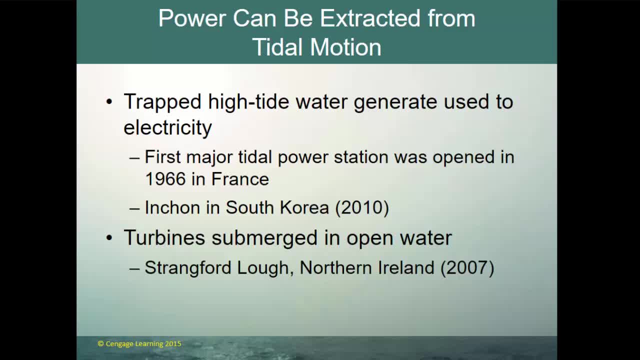 And the first major tidal power station was opened back in the 1960s, in 1966. We've also seen them in South Korea. Essentially, they submerged turbines in open water to allow the tide pushing back and forth, as they did in Northern Ireland, to drive those turbines. 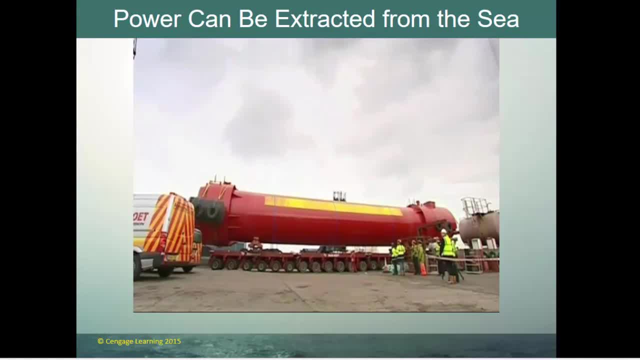 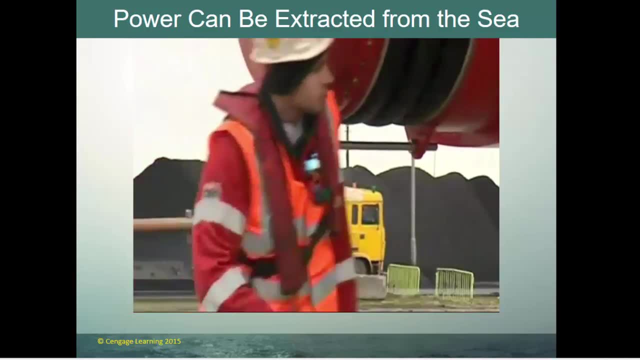 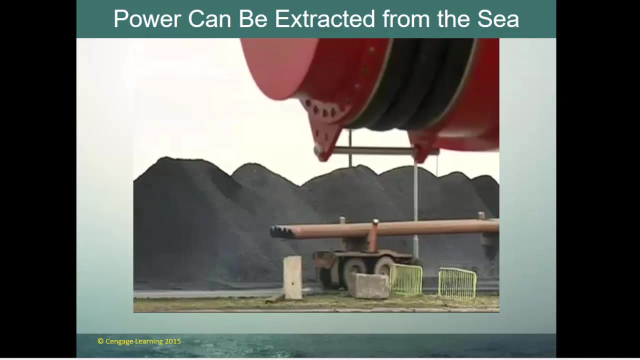 Inch by inch, a new source of energy is emerging the size of a submarine Here at the dockside at Leith near Edinburgh. a vast wave power machine Nearby mounds of coal. It was coal that fueled the Industrial Revolution. Could sea power be next? And this component is now being lowered. 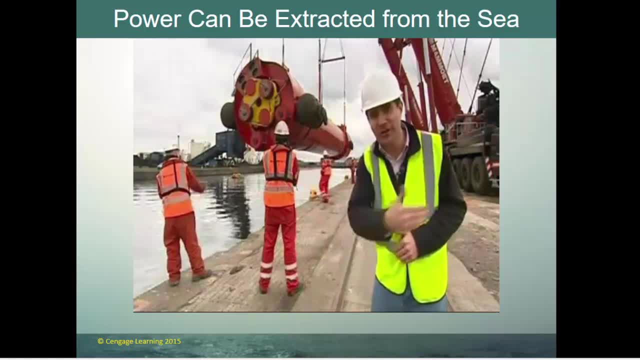 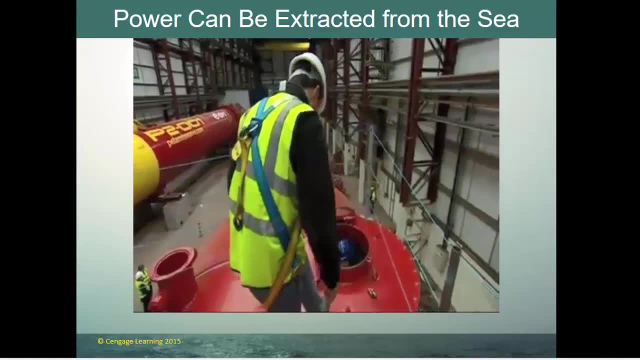 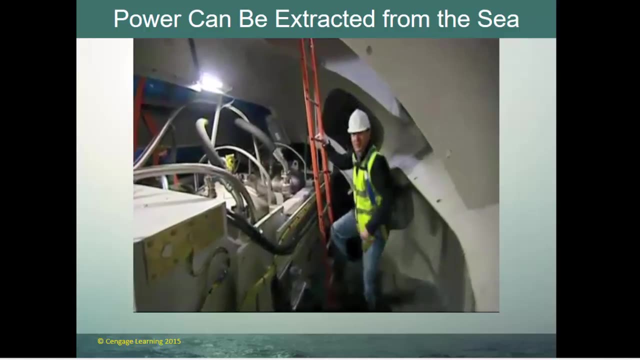 into the sea, An operation that will have to be repeated thousands of times at the start of what's been described as a new era of harnessing the power of the sea. So, to follow on, in the assembly hall, I was given the chance to see inside, down through the hatch. It's just like being inside a. 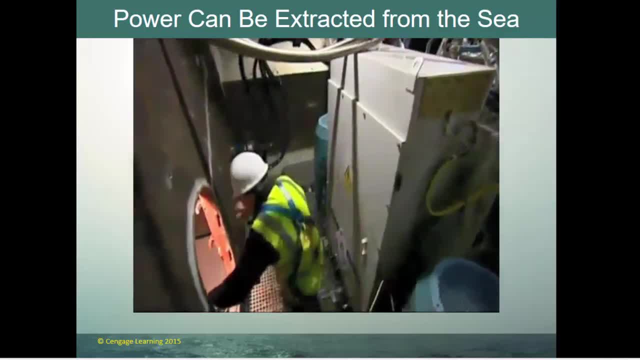 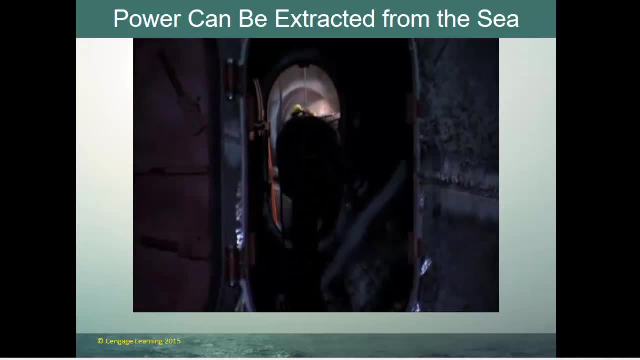 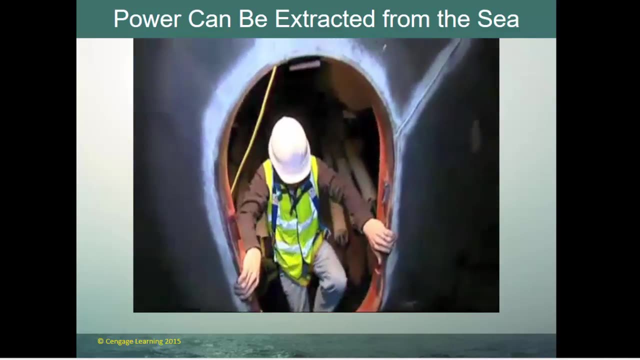 submarine. It's a strange new technology. So far it's cost some 40 million pounds. Out at sea- there'll be no one in here to feel the rocking of the waves, And here, at the end of this giant cylinder, is where they actually generate the power. Let me show you how that's done. 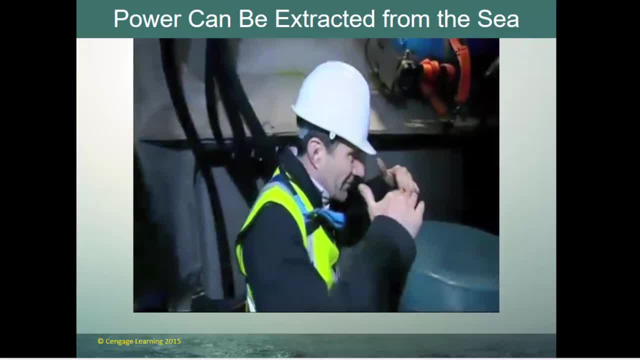 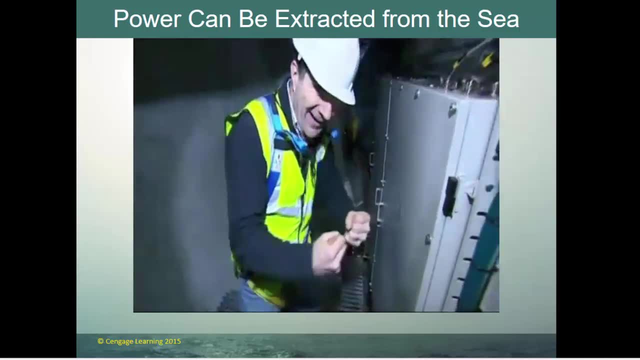 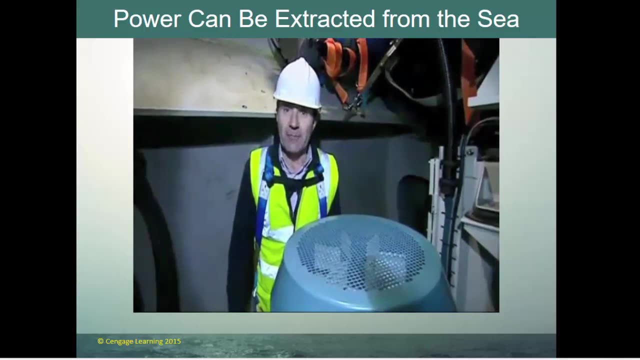 Every time a wave passes along this system, the cylinders move, And where they're hinged, there are these huge hydraulic pumps like bicycle pumps, And that captures the energy of the waves. It's channeled to the world into a generator like this and ends up producing electricity. Cables will bring the power ashore, But what if there are no waves? 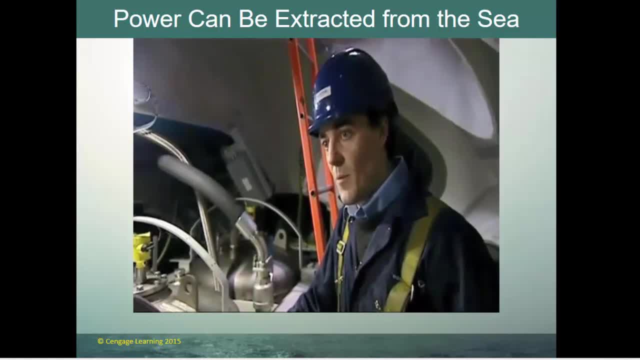 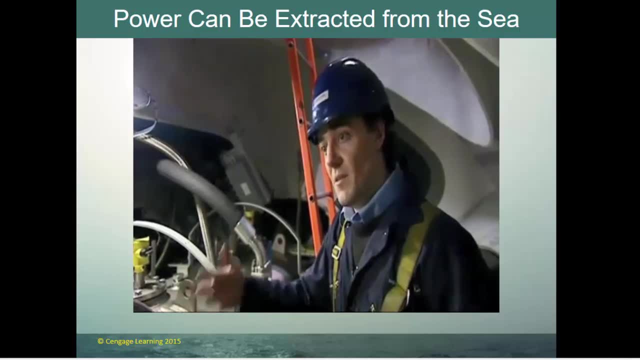 This thing will be useless on a flat day. On a flat day, we won't produce any power, That's right, But the important thing is the contribution on average over the year. Every megawatt we generate is a megawatt that doesn't need to be provided by fossil fuels. 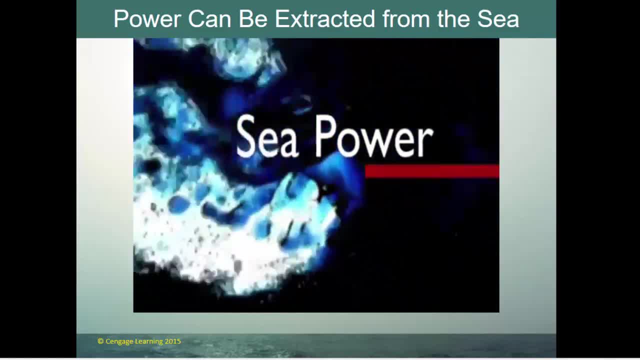 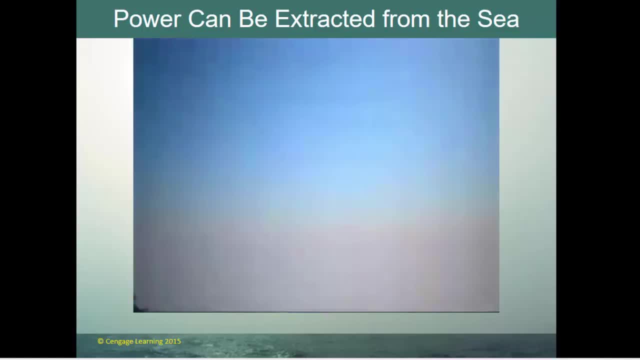 This plan to harness the power of the sea is the largest of its kind in the world. Electricity for 750,000 people. 1,000 homes could be produced. if all the projects go ahead, That's 1.2 gigawatts. What a conventional power station generates A bold ambition from the official agency leasing out 10 areas of seabed. 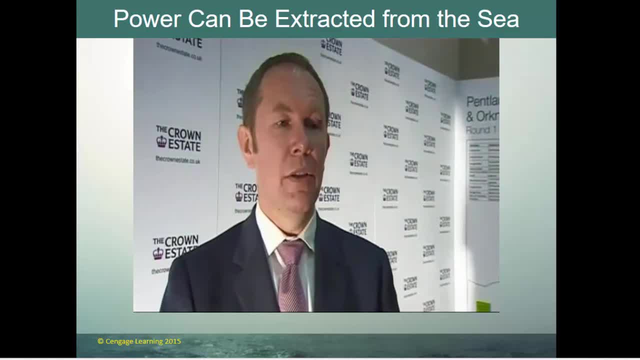 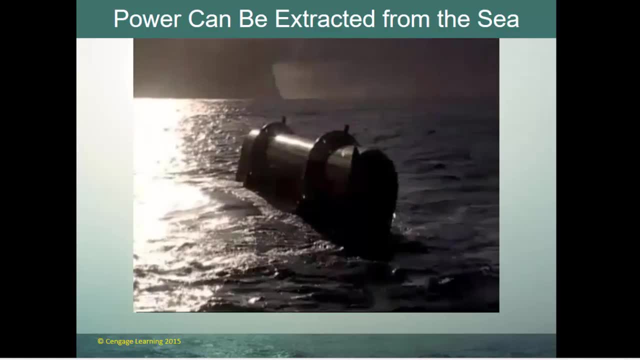 This is a very important day. What we've actually done is taken a very big step to making a new technology, a renewable energy technology, wave and tidal- commercially deployable on a grand, on a big scale. The designs range from wave machines swaying in the swell 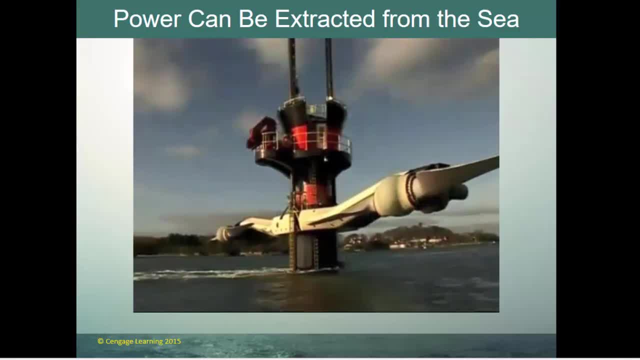 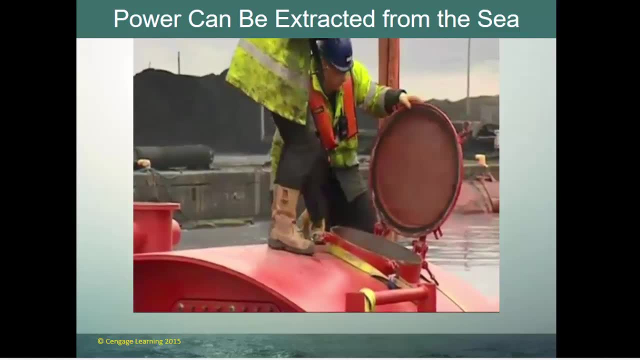 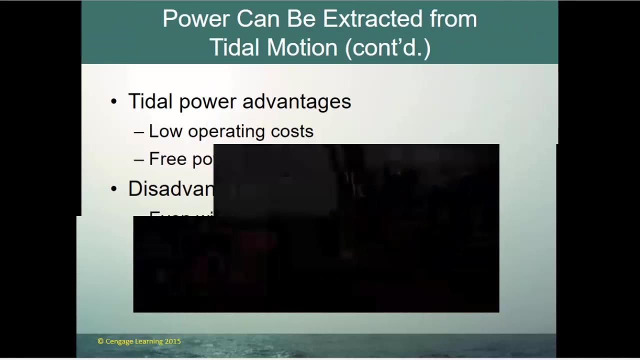 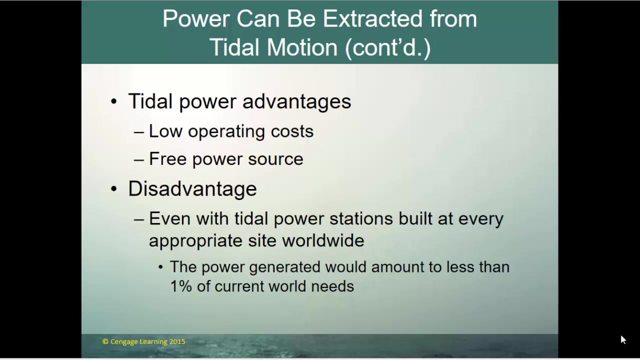 To giant turbines spinning in the tides And huge propellers harnessing the currents, Another component is launched. There may yet be unexpected costs or challenges. It's still early days, David Trukman, BBC News in Leith. So there are some very exciting possibilities with tidal power. They have very low operating costs and, of course, it's a free power source. 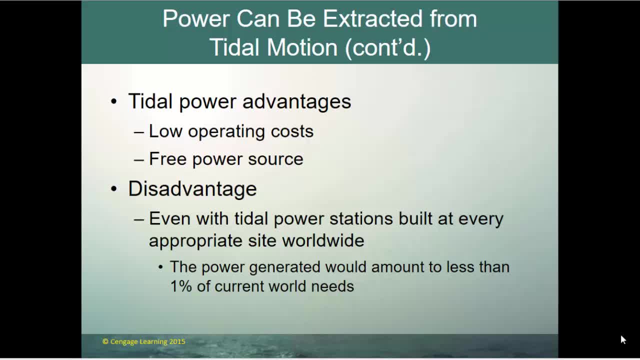 Now the low operating cost is to operate the machinery, to build it, to put it in place. That can be expensive. The biggest disadvantage of tidal power is that even if you built stations in every place in the world where you could use them, you probably would only generate about 1% of the current world needs of energy. 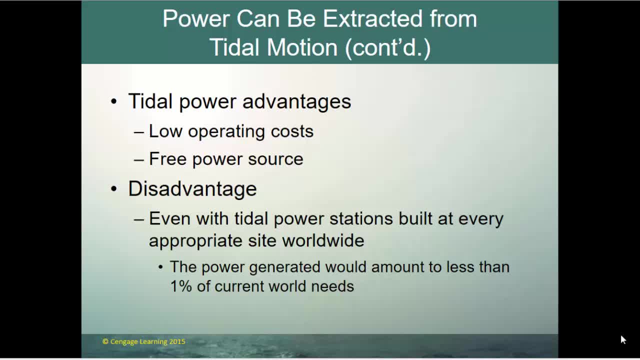 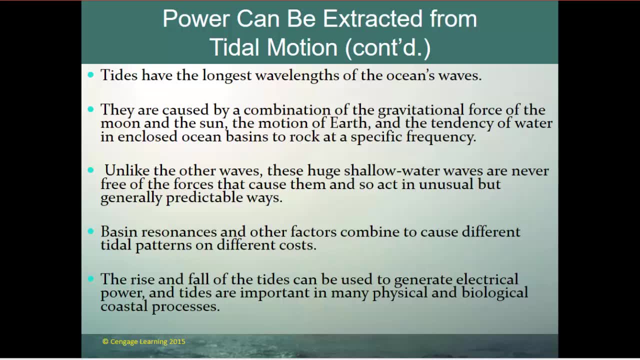 So it's not necessarily a worldwide solution to power generation, Although it may be one solution. So just to summarize, Chapter 10.. Tides are the longest of the ocean's waves. They are forced waves, Forced by a combination of gravity from the earth and sun. 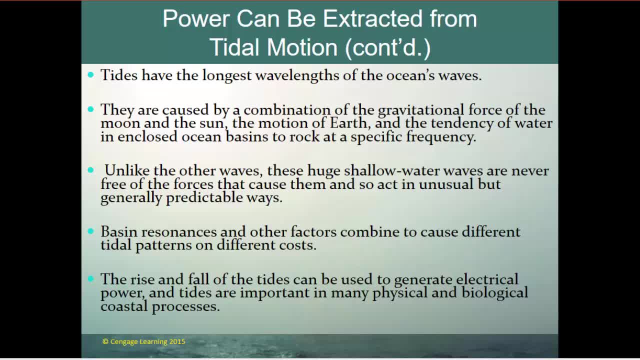 And they're affected by the motion of the earth, the contours and the shape of the ocean basins and a couple of other factors, and how water tends to move within ocean basins and rock at a specific frequency. All those things are part of the dynamic theory of tides. 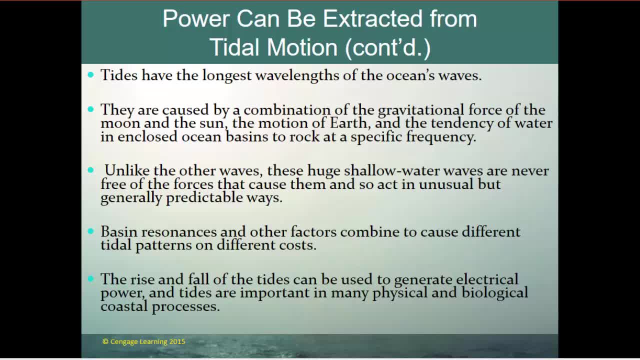 Unlike other waves, these massive shallow water, very long wavelength waves are never free of the forces that cause them. So they act in an unusual but generally predictable ways. And again that's that tidal power, Again that's that dynamic theory of wave prediction. 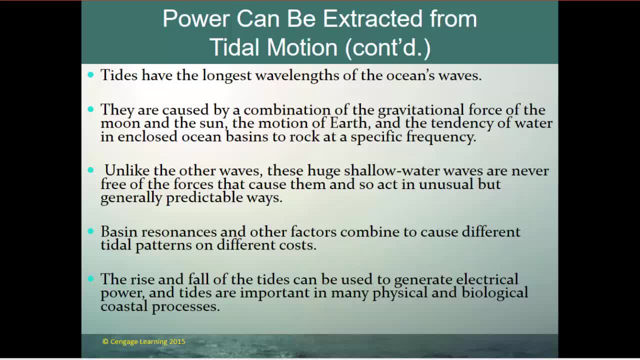 And basins, as we learn, can resonate. Basin resonances and other factors combine to cause different tidal patterns at different coastlines. Remember you have diurnal tidal patterns like an enclosed basin, Up down, One tide high, one tide low each day. 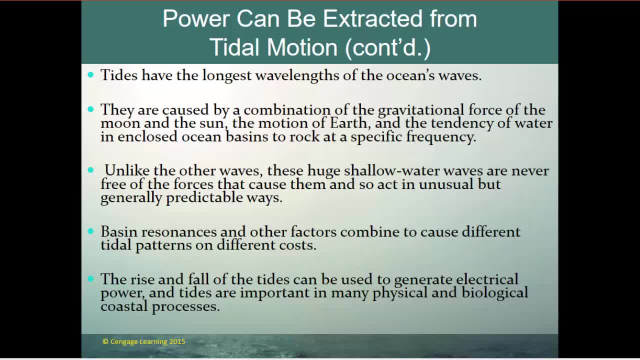 Other coastlines. more open coastlines have semi-diurnal And then others have mixed tides, So different basins have different types of tides And the rise and fall of tides. And the rise and fall of the tides can be used to generate electrical power. 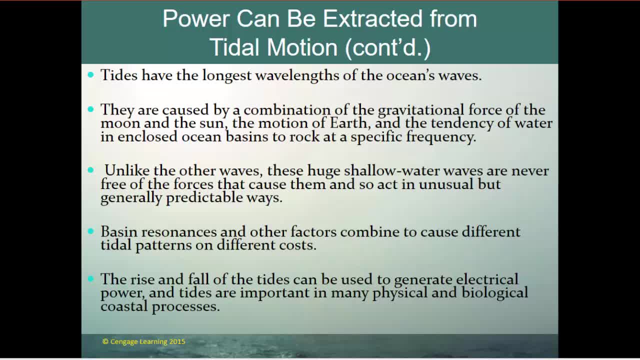 And tides are very important in many physical and biological coastal processes. All right, that is going to wrap up chapter 10.. We will see you, or at least we'll be together again for chapter 11.. 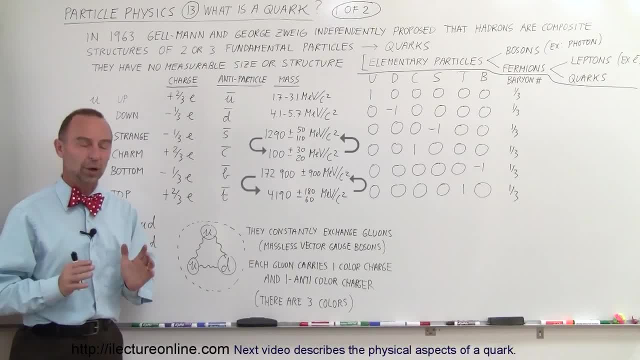 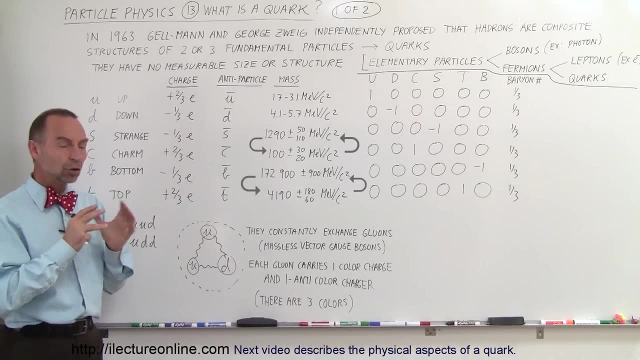 Welcome to Electron Line, and now we're going to talk about the quark. So what is a quark? Where did it come from? Why do we know it exists? Well, there's already a suspicion that nuclear particles, neutrons and protons the ones that make 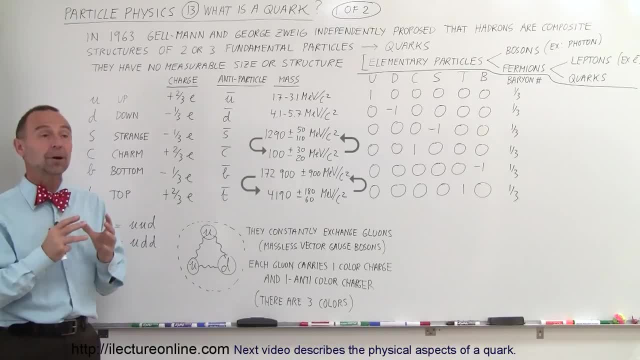 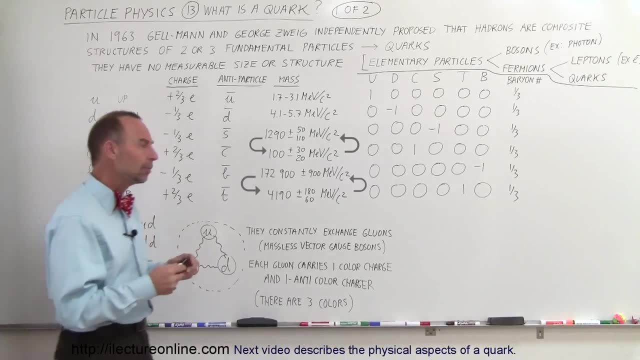 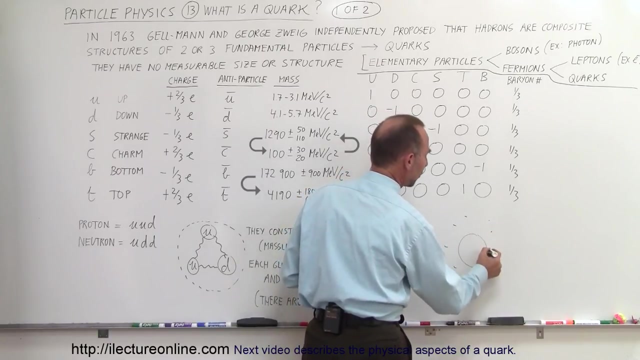 up the nucleus were not what we would call elementary particles. They thought they may be subdivided into even smaller particles. and the reason why they had that suspicion is because sometimes, when you have a nucleus- so nucleus containing protons and neutrons, with electrons zipping around at very high speeds and 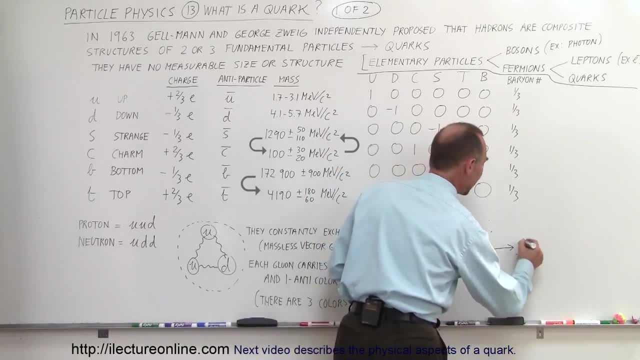 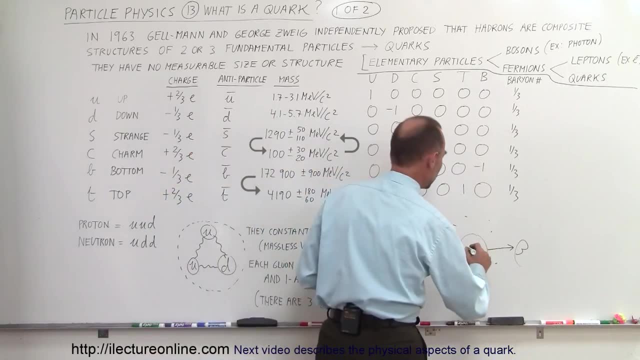 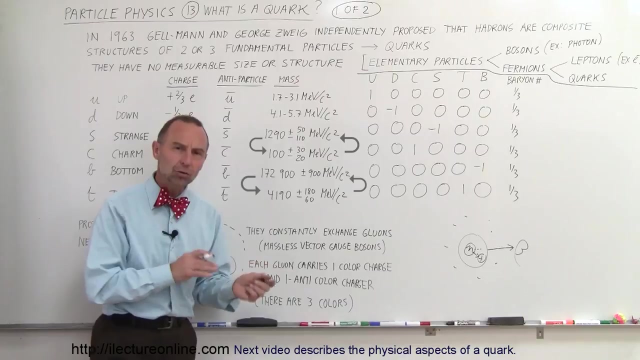 every once in a while, a nucleus would shoot out a beta particle, and a beta particle is actually an electron- An electron from the nucleus and what happened was a neutron would release an electron and it turned itself into a proton. And if neutrons and protons were elementary particles, that would be a